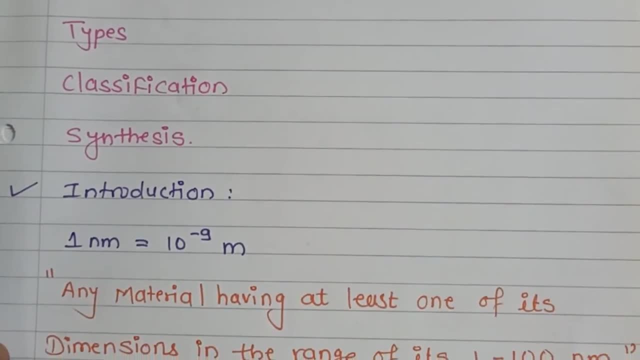 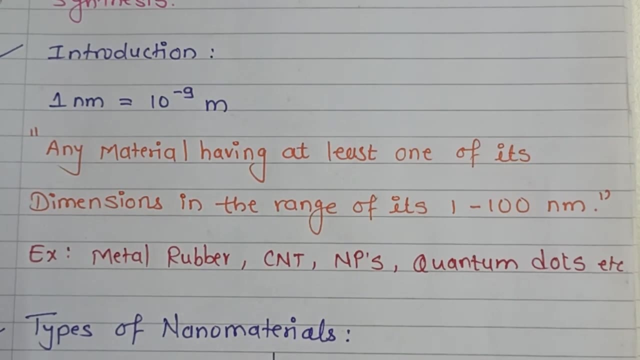 chapter. Okay now, after understanding the brief part of the nanochemistry part, now we move towards the introduction part. So what is the introduction? So introduction is the introduction of the nano materials Here. nano is nothing but what we are going to be learn: the nano materials, Now your. 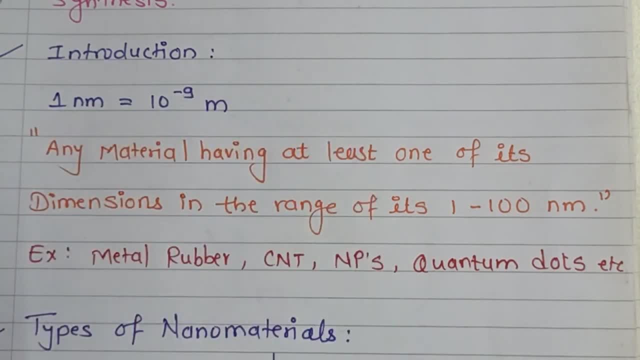 nano means what? the nothing but the one nanometer is equal to what your 10s to minus 9 meter. Now these things are going to be known to everyone. Now, 1 nanometer is nothing but what your 1 billionth of meter and the another definition for the nano material will be. it is a any material having at 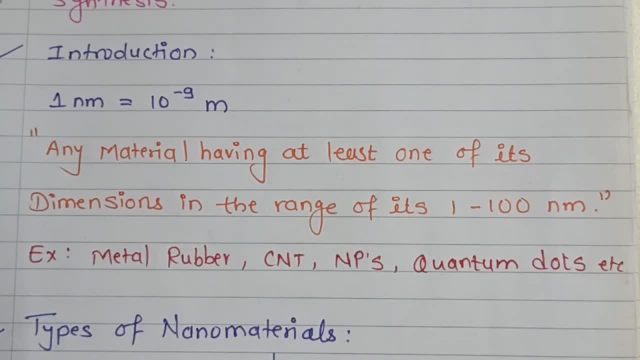 least one of its a dimension in the range of 1 to 100 nanometer. So we can say, for example, suppose you have the 100 crore rupees, so from that, if i am going to be considered, the one rupee means your one nanomaterial. so these 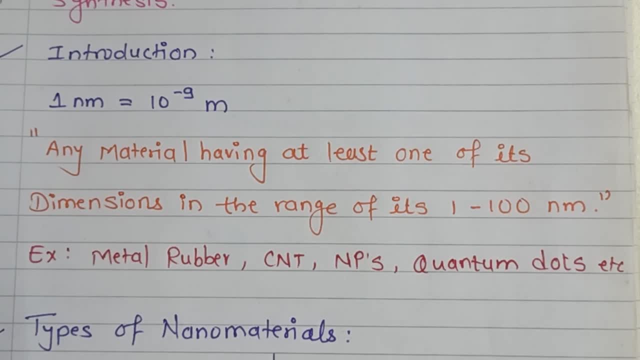 are the actually meaning of your nanomaterials. so basically this term nanomaterial will be first time introduced by the norio taniguchi in 1974. okay, so also these words- nanos words- are coming from the greek word- means dwarf. dwarf means it's actually very small, means miniature scale. 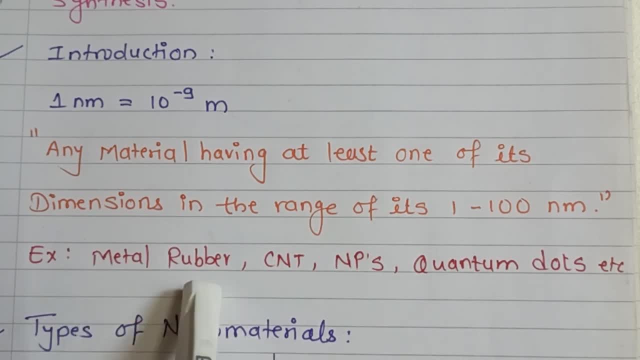 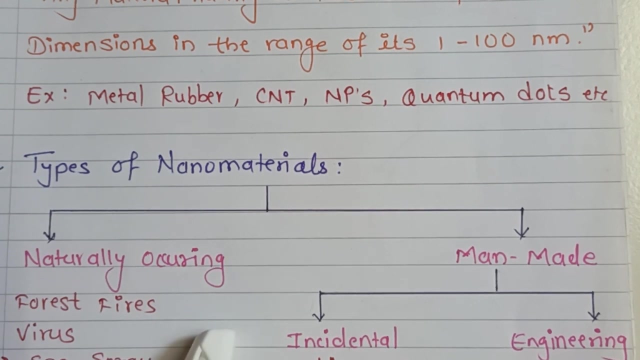 so, for example, in the nanomaterial we can consider the metal rubbers, carbon nanotubes, nanoparticles, quantum dots and etc. okay, so these are the actually main reason, that why we have to learn the nanomaterials. so further we move towards the types of the nanomaterial. now the types of the 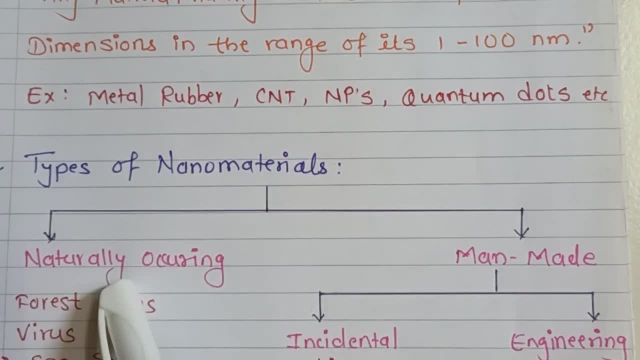 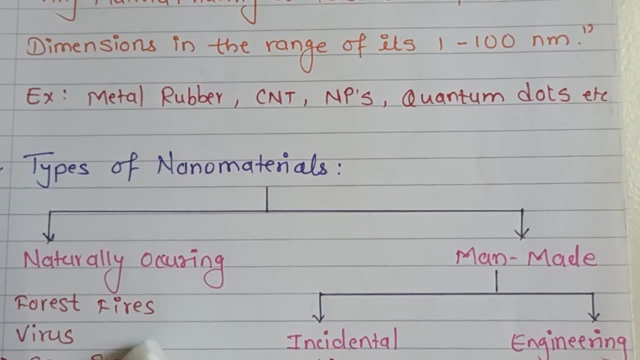 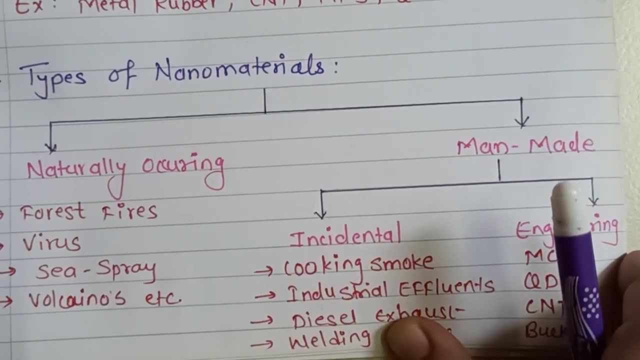 nanomaterial. basically, they are actually two types. first one will be the- they are the naturally occurring, whereas the second one will be the man-made. now naturally occurring nanomaterial means, you can say, the forest fires, virus, apart from that, sea sprays- and the fourth one will be the volcanoes. okay, so these are the. 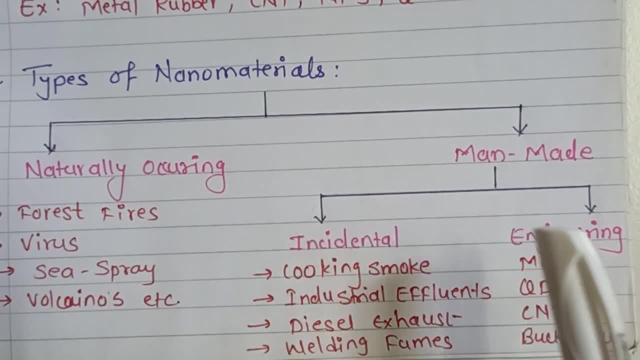 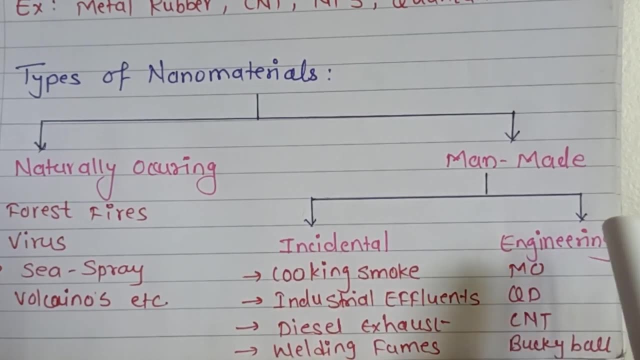 actually part of your what? naturally occurring material, then man-made. again further classified into the two types, one will be the incidental and another one will be the engineering. man-made means here that we are going to be synthesize the nanomaterials by artificially, so incidental. 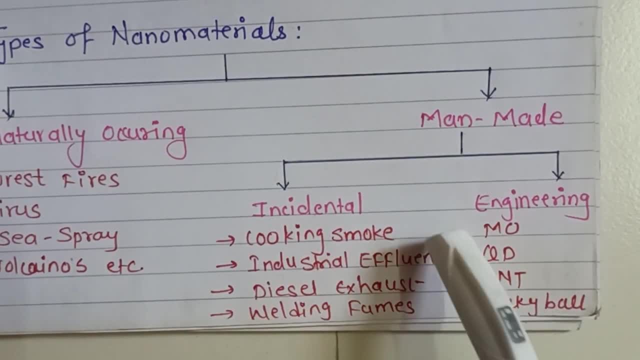 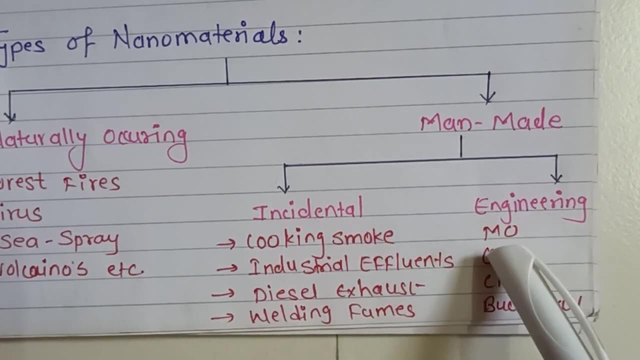 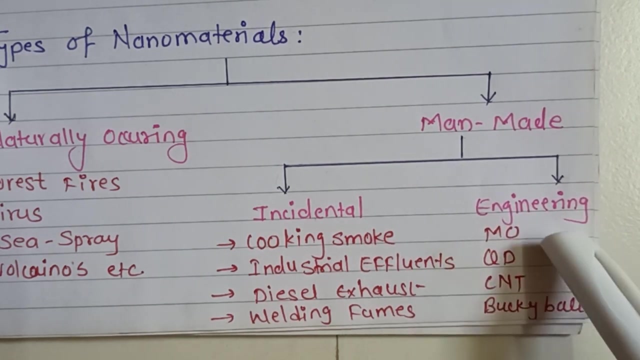 means by incident they are going to be generating, like your cooking, smoke, industrial effluents, diesel exhaust and the welding fumes into metal. because engineering nanomaterial means these are the what you are: quantum dots, carbon, nanotube, bucket balls, okay, and the metal oxides, mo kmed away: metal oxide, qd, quantum dots, cnt, carbon. 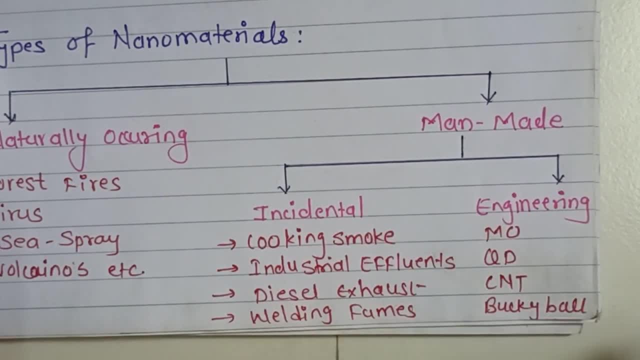 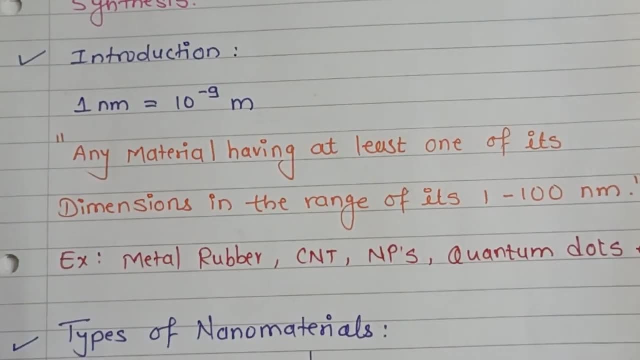 nanotube and the bucket bottles. so these are actually some of the types of the nanomaterial which is going to be studied in the throughout the chapter, okay, but apart from that, okay, there will be the another types of the manom centimetrick also we are going to be studied in the nano chemistry. that 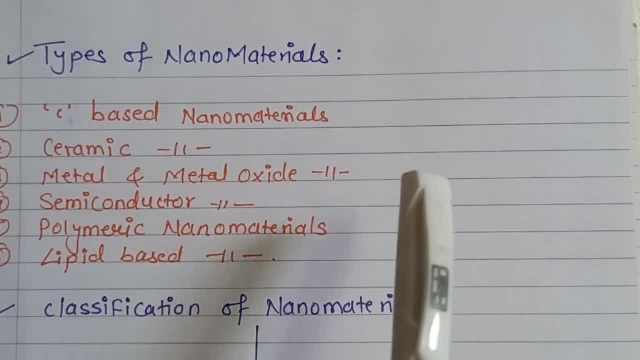 carbon-based nanomaterials. so nowadays everyone is going to be more focused on the carbon-based nanomaterial, then ceramic nanomaterials, metal, metal oxide nanomaterial- again it is also very interesting part semiconductor nanomaterial, polymeric nanomaterials and the lipid-based. 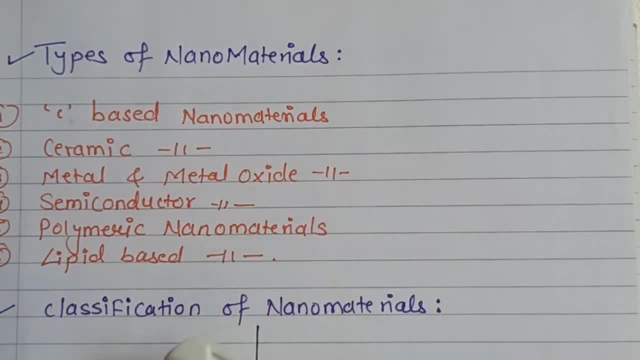 nanomaterials. so, apart from the naturally occurring and the man-made, these are the some of the types of the nanomaterial which are going to be more fascinated area towards the research and development. okay, so now, after understanding the all the kinds of and all the types of the 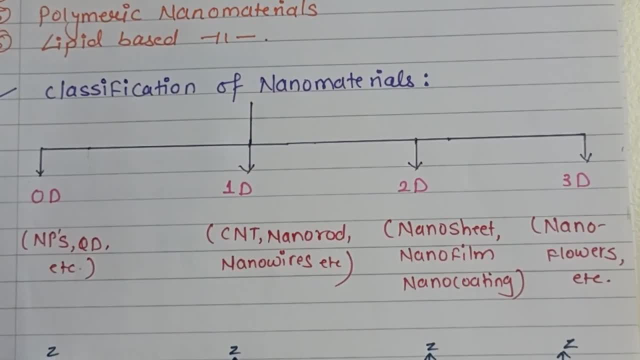 nanomaterial. we further look into the. what are the classification of nanomaterial? now, these classification actually based on the, your dimension. now, what is the dimension? dimension with respect to a, x, y and the z axis. so, depending on the x, y, z plane they are going to be classified into mainly. 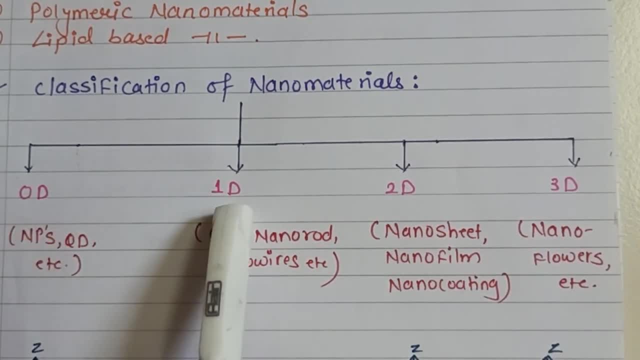 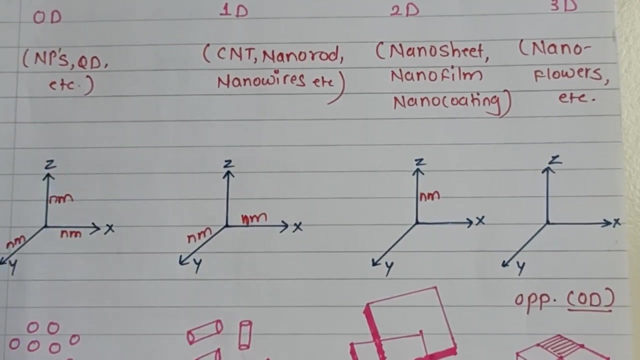 four types: the first, zero dimensional, second, one dimensional, third, two dimensional and fourth one will be the three dimensional. okay, so, as you are going to be look on to look into here in the zero dimensional I am going to be draw the diagram: the x, y and z plane. so if you can see in the x, y, z axis, all, the axis means all. 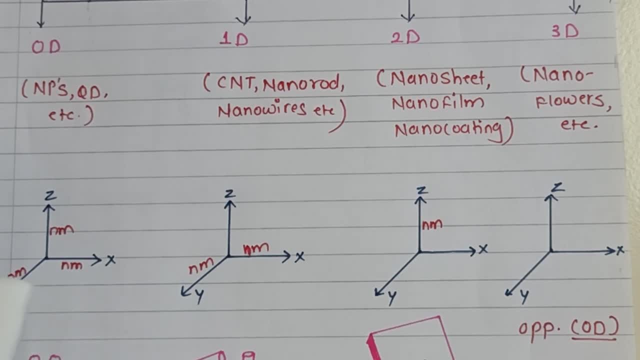 the plane are going to be confined to the nanomaterial scale. so we can say it's a zero dimensional so, in which the movement of the electron is going to be confined in all the three dimension. so we say here we will say zero dimensional, for example, you 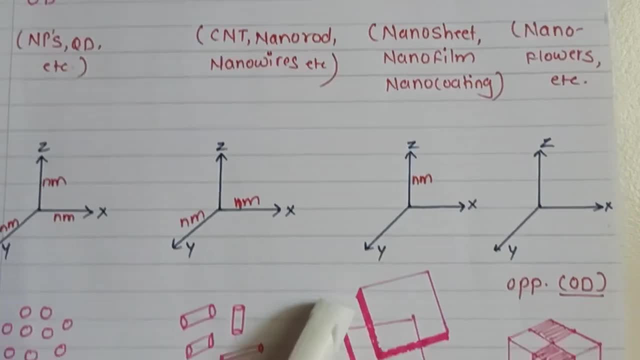 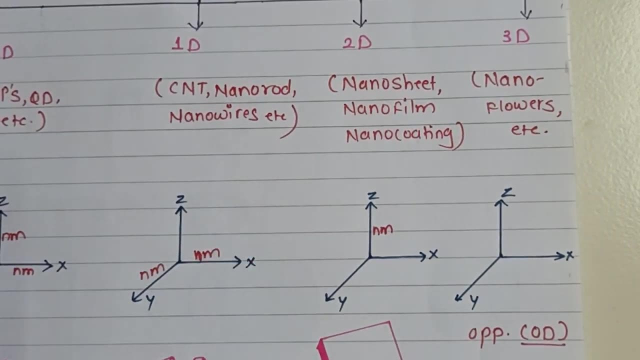 can say the nanoparticles, quantum dots, etc. so look into here. these are the actually nanoparticles diagram. okay, now we move towards the next part will be the your one dimensional. now, one dimensional means what? what is the meaning of the one dimensional over here? as you can see in the 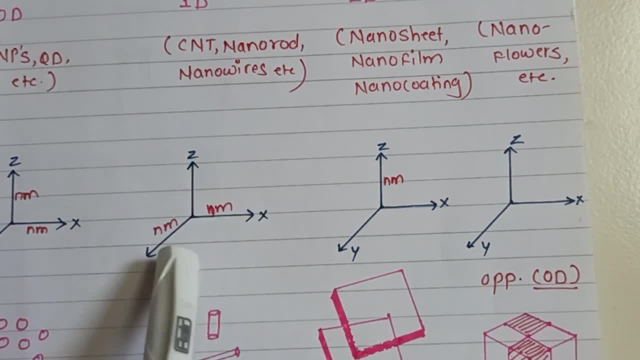 diagram, the x, y, z plane. in this, out of the three plane, only the two plane in the nanometer scale, whereas the one of the scale means one of the plane has to be in the larger amount in the large scale, whereas the x and y will be confined to the nanometer scale. so we say here, we say one. 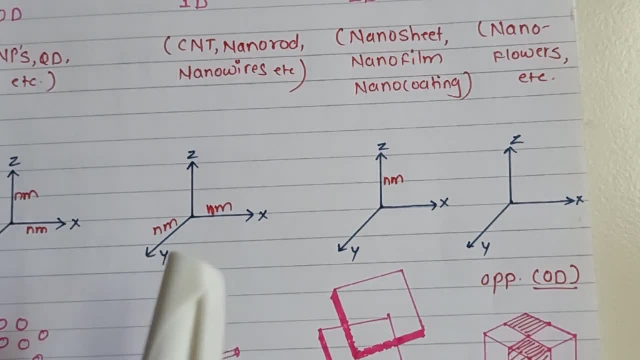 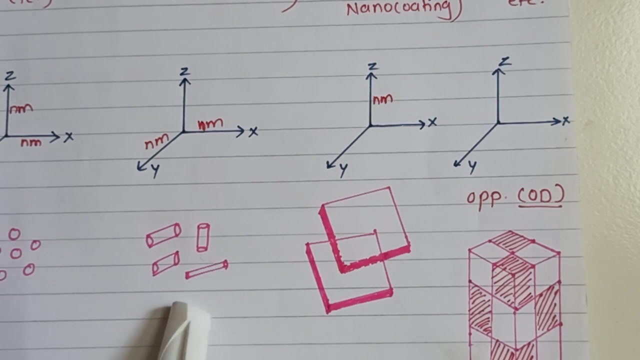 dimensional. so the one dimensional in which the electrons can only move freely into the any one direction. so here it can move freely on to the z direction. so we say here we say student one dimensional, for example, carbon nanotubes, nanorods or the nanowires, etc. so these are the actually 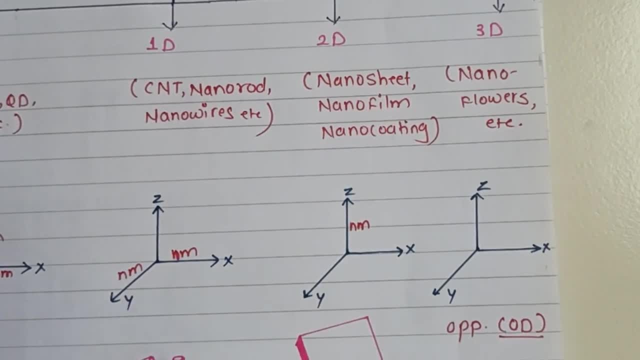 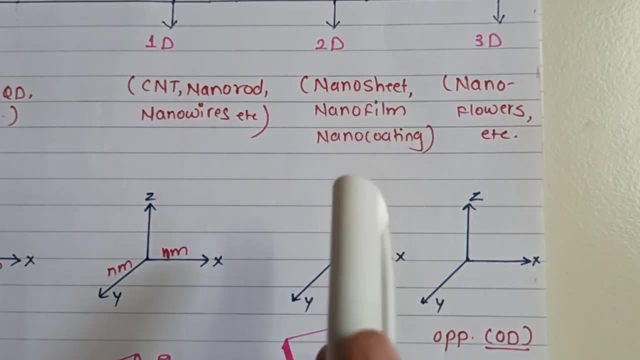 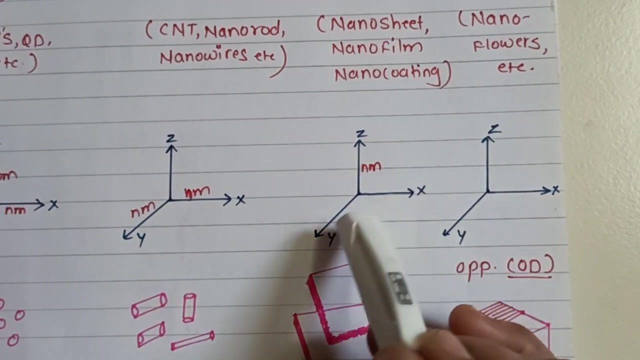 what your example are: the 2d then, sorry, 1d. now we are going to be move towards the two dimension. so in the two dimensional in which the free electron can move into the, any two plane means into the x and the y plane. so, if you can see, the x and y plane will be the free. 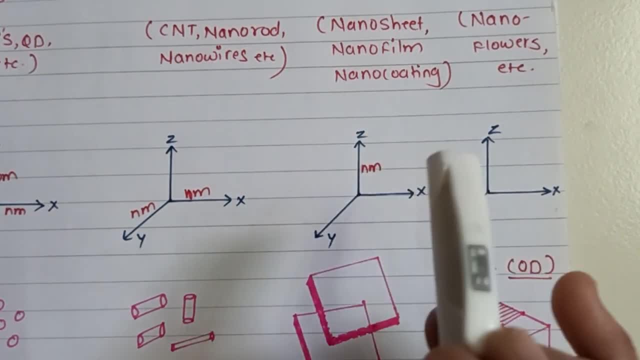 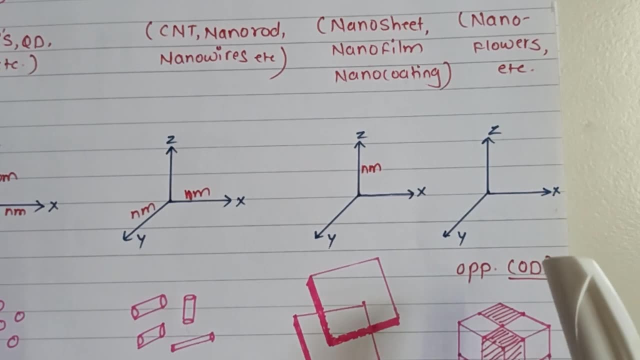 for two electron move here and there, whereas the one of the plane has to be confined to the nanometer scale. so here we keep the z axis as nanometer scale, whereas the x and y will be the larger in scale. so we consider this example in this nano sheet, nano film. 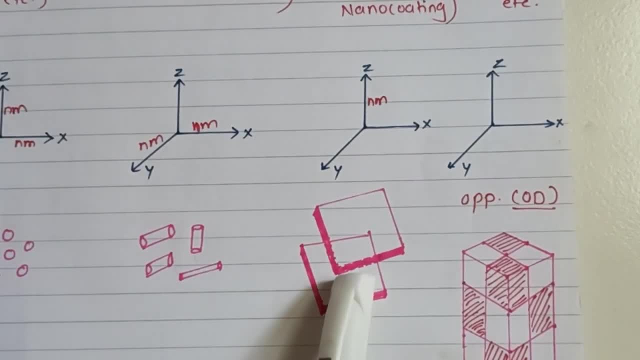 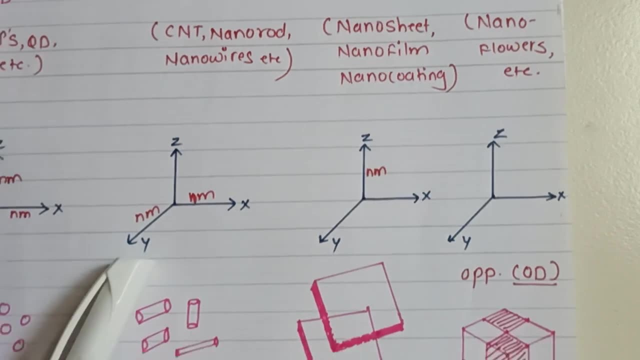 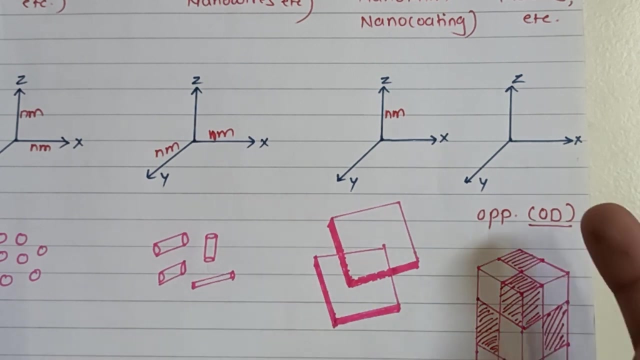 and the nano coating. so you can see these are the nano sheet or nano coating. we can see now, last but not the least, the three-dimensional example in nano flowers, buckyballs, etc. so here, what happens into the three-dimensional nanostructure material built a nanoparticle as a building block in which the 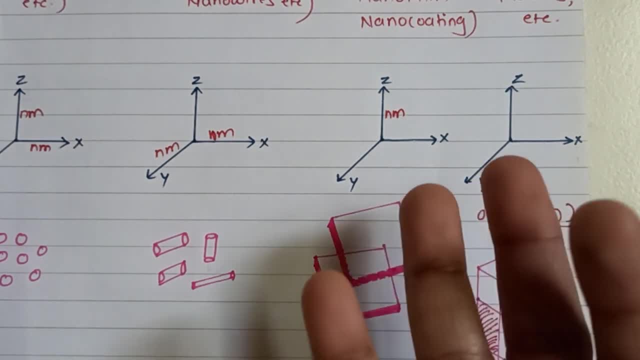 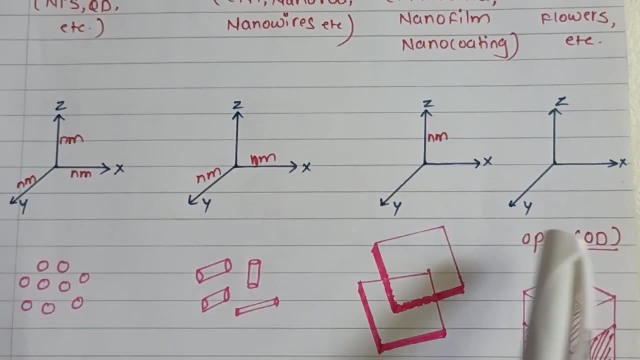 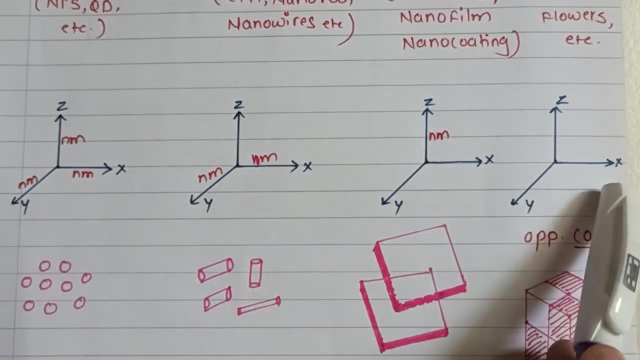 free electron can move in any direction of the xyz plane. so here, all these planes are free. they are not confined to the nanometer scale. so it is exactly opposite to zero dimensional, whereas the xyz plane in the zero dimensional, they are confined toward the nanometer scale, where they 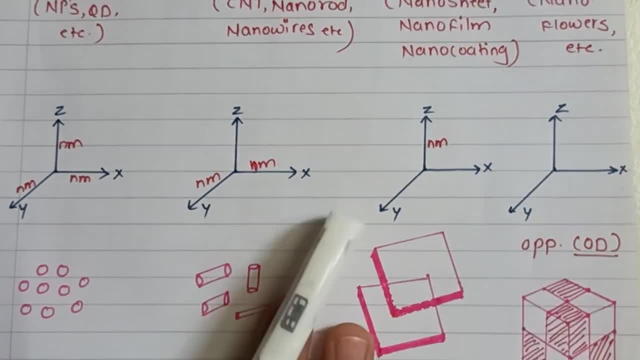 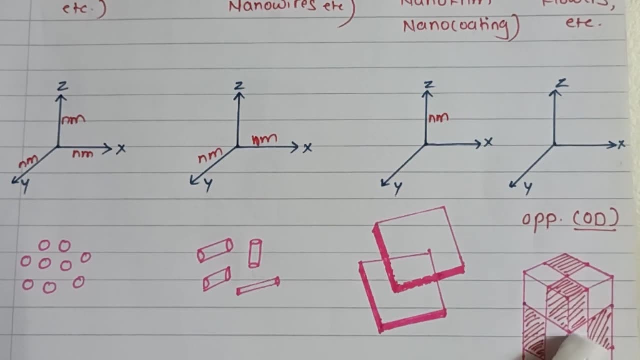 doesn't confine to the nanometer scale. so, exactly opposite to that, we call it student three-dimensional. what nanomaterial? so, as you can see, these are the block diagram for the, your nanomaterial, or you can say, as an example, nano flowers. okay, now, after understanding all the classification in based: 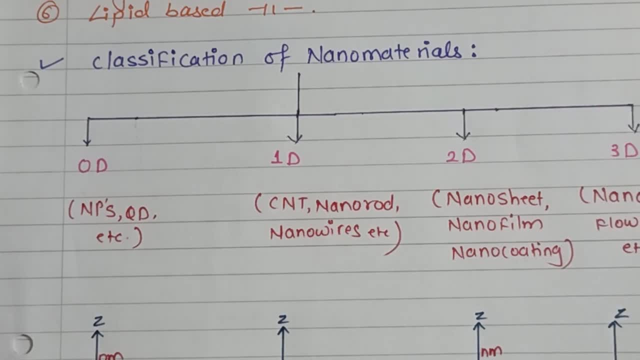 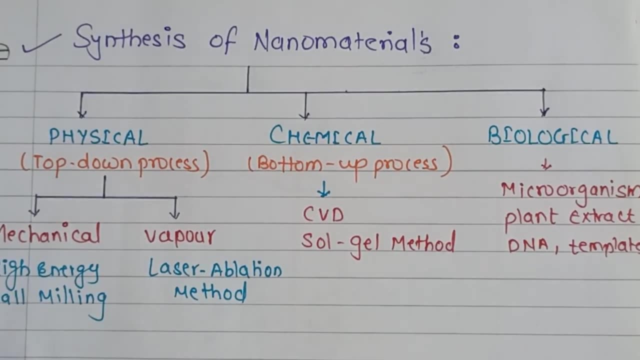 on the- your dimension. we move towards the, our next part of your outline of the course, that how we are going to be synthesize the nano material. so these are the actually basically most important part of your nano chemistry. so we can say hard because, end of the day, what we are going to be interested in, that how we are going to be. 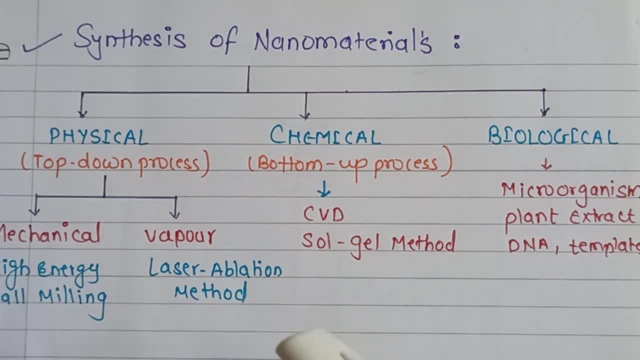 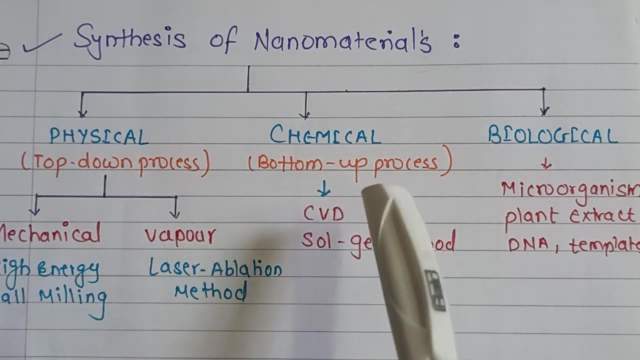 synthesize it. so, basically, the when you are going to be synthesize the nanomaterial, there are basically mainly two approach. they are going to be followed. so those two approach are here: top down and bottom up approach. okay, but apart from that, we are going to be synthesize, okay, nano material depending upon their mechanism and depending upon 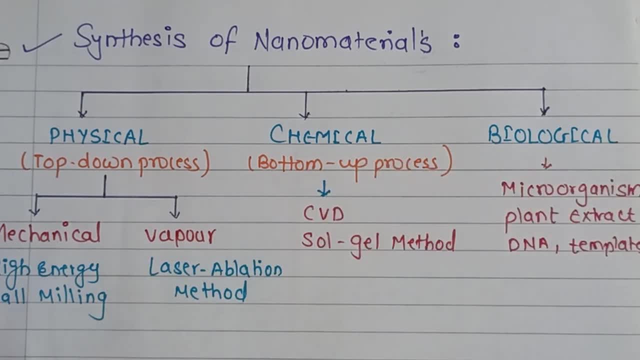 their process. they are the only classified into mainly three parts. so in that your first part will be physical method, second chemical method and third one will be the biological method. so physical method will be the part of top down process and the chemical method it is a part of bottom up. 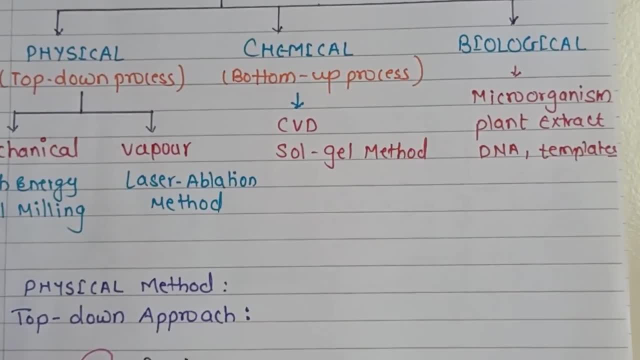 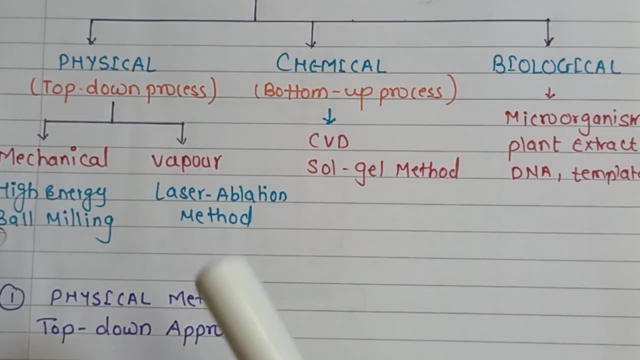 process. okay now what is happening? you over here, just take a look now. physical method is nothing but what should follow some of the mechanical attrition in this process, and then that has to be by followed that particular process. you are going to be making the nano material now again in the physical. you. 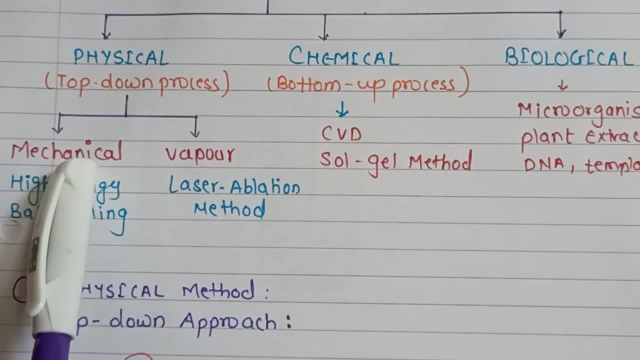 could see over. here they are: follow the two process. one will be the mechanical and where is the second? one will be the vapor. in the mechanical, we are going to be learn in this session high energy ball milling method, and in the vapor, we are going to be study the laser ablation method. 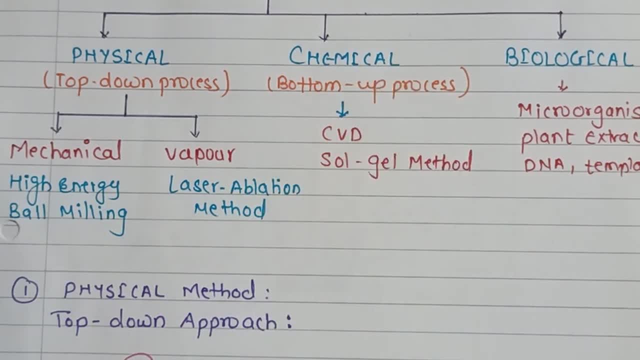 further in the chemical we are going to be study over here the mainly two method. the first method will be over here student, that will be the cvd, cvd- come at the happy with a student- chemical vapor deposition method. and the second one will be your soul gel method. so, apart from this bottom, 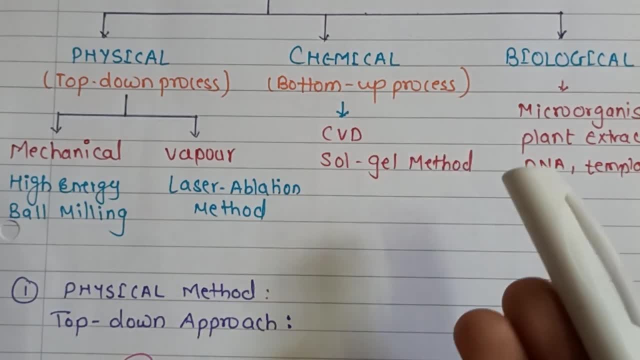 up process in cvd and the soldier method. there will be the another method also we are going to be considered in chemical, that is, a hydrothermal method, co-precipitation method, solar thermal method, and then we are going to be studying the chemical and the second one will be your. 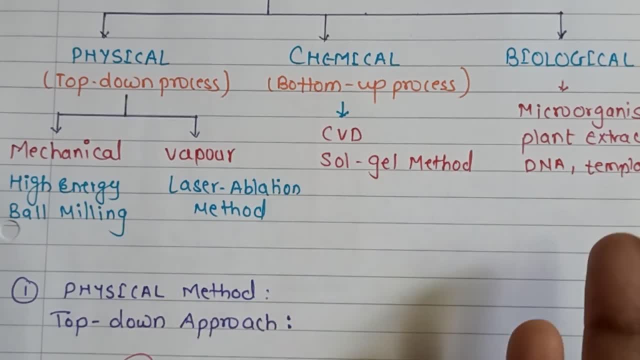 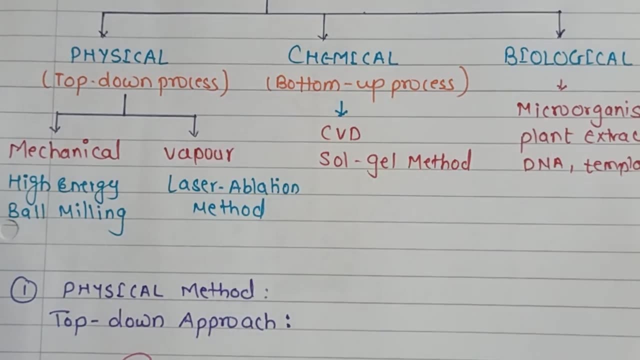 method. I know thermal method but we are not going to be study. there are various kinds of the processes in the chemical method but we are going to be study in this session only the two method, that will be the cvd and the soul gel method, and third one will be the biological method. now 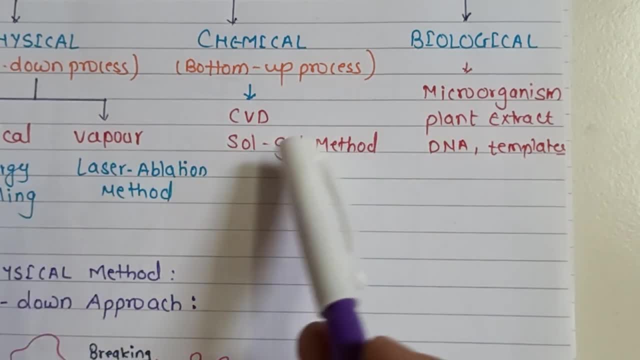 biological method instead of we are not going to be- is any physical and the chemical process. we directly take over your biological ingredient and that biological ingredient has to be reacted with. the nanoparticles means your metal salt and metal oxides and they are going to be converted into the. 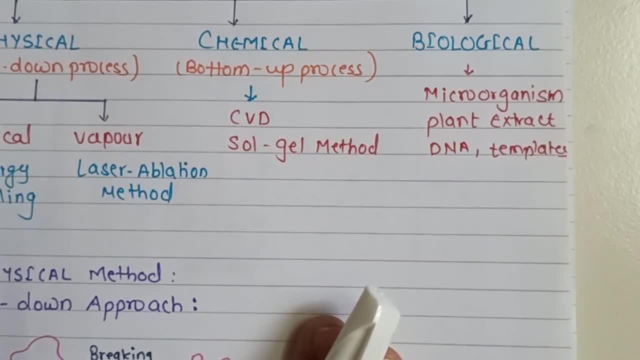 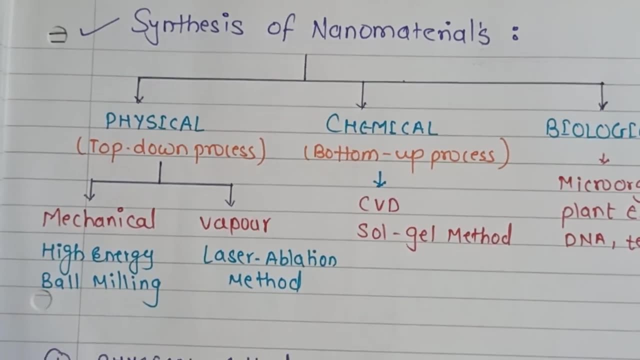 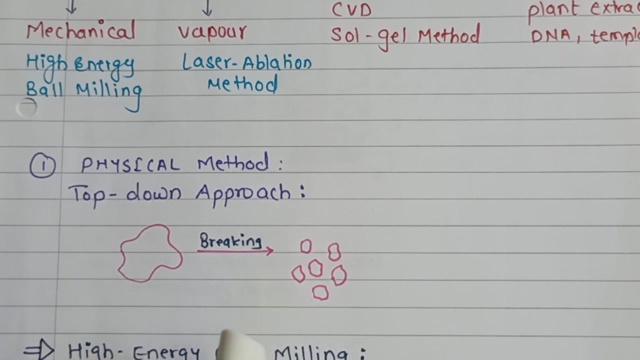 finally, nano powder. okay, so these are the mainly three main processed that how we are going to be synthesized. the nanomaterials, okay, so we look into their first and physical method. so take a look. so physical method, actually basically the top-down approach. top-down approach means that we are going to be 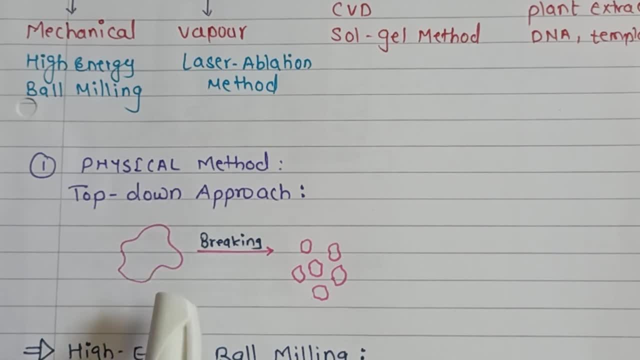 considered over here the larger molecule. okay, so that larger molecule has to be breaking down. okay, and we will get over here the smaller molecule, which is the nanostructure. so the process by which the more an atom occurs in the course of the 663 is the smaller molecule, or the process we will get over here the smaller molecule, which is the corporations. so the process used here is called the fifth line. 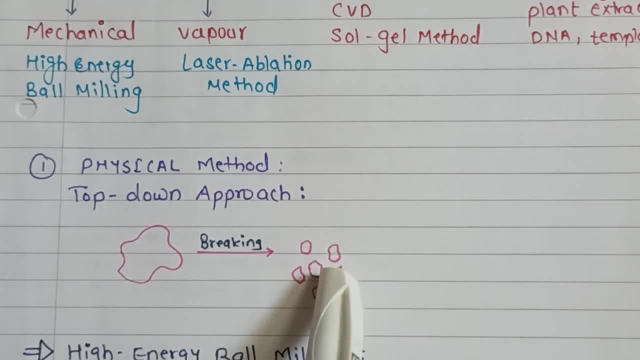 structure. so the process of making what nanostructures, starting with larger structures okay and breaking away to the nano side, is called basically what your top-down approach okay. so in the top-down approach, for example, we can say: the ball milling, epitaxy, lithography. these are the some of the example of 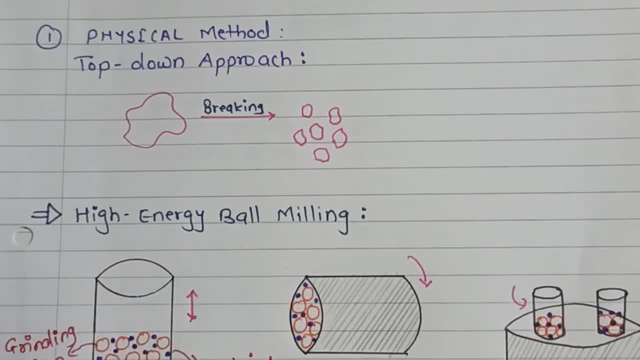 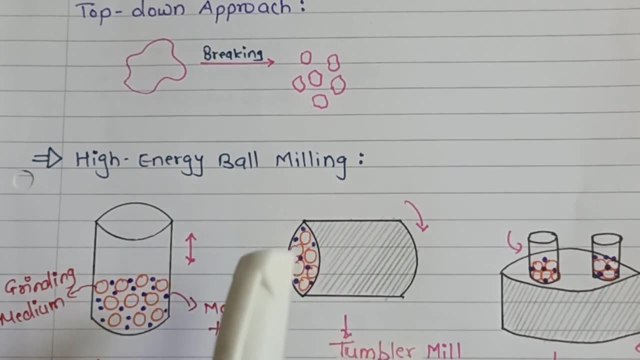 your what top-down process. but in this we are going to be study what your high energy ball milling, not just take a look, a high energy ball milling up, go yeah. basically there are the three kinds of the processes. so it is actually one of the simplest ways to making the nanoparticle of some metals. 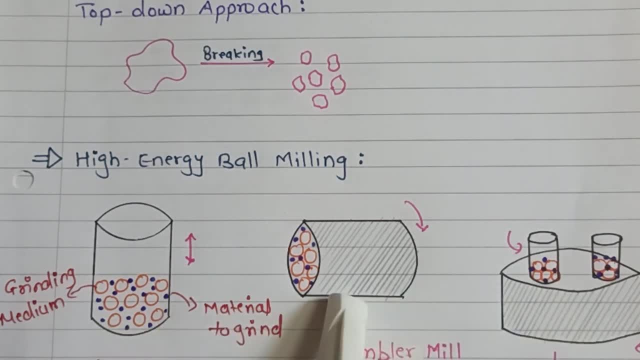 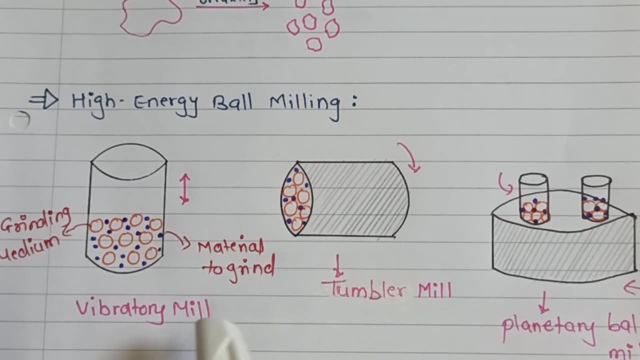 or we can say the alloys in the form of powder. so there are many types of the mills, okay. so, as you can see in the diagram, so these are the all the types of the mills, like your planetary mill. okay, these are the vibratory mill and these are the tumbler ball mill. okay, so, in the all the process, okay, the main. 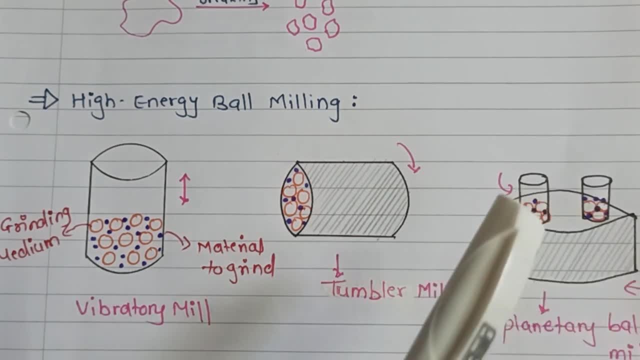 principle of this process will be the grinding: grinding of your sample material with the help of the what your metal balls or stainless steel ball- we are going to be used and we are going to be making the finely coarsed powder which we have to make here. so these are the actually main purpose of this. 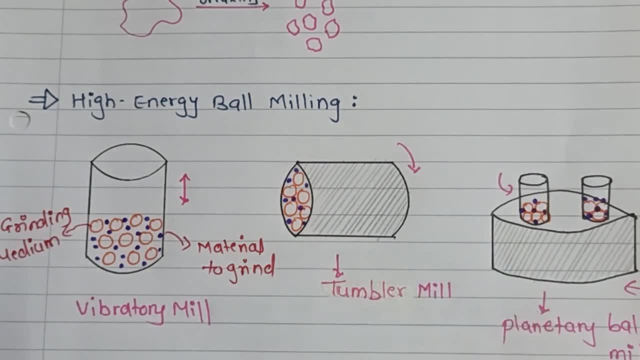 technique. so, as you can see here in the what, when, in when, the containers are going to be rotating. so basically what happens here, such type of the containers will be there. for example, consider: these are the actually container. so in that container, what we are going to do, we are going to take the stainless steel or the 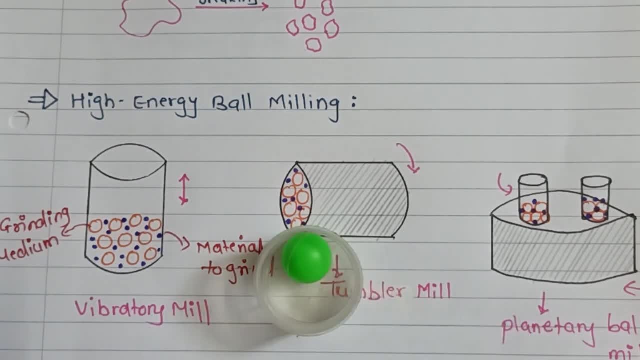 metal body rigid mass and we are going to take the stainless steel or the metal ball. if they have plastic ball, orельзя, put free ball. and then we are going to put types of the materials, our founded esimerk lecture. they are not in question. 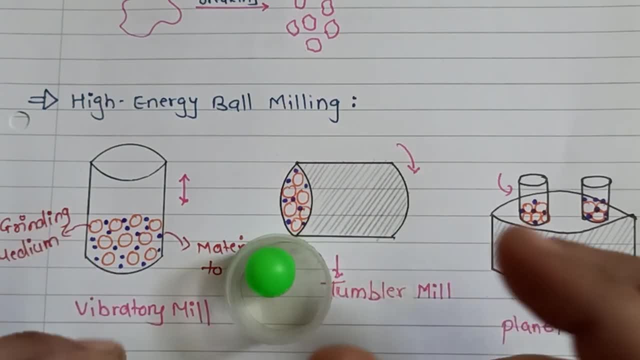 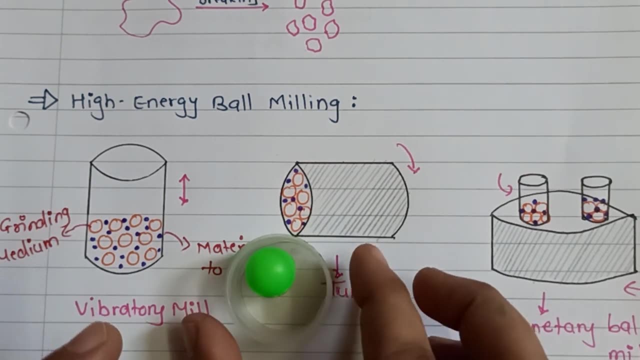 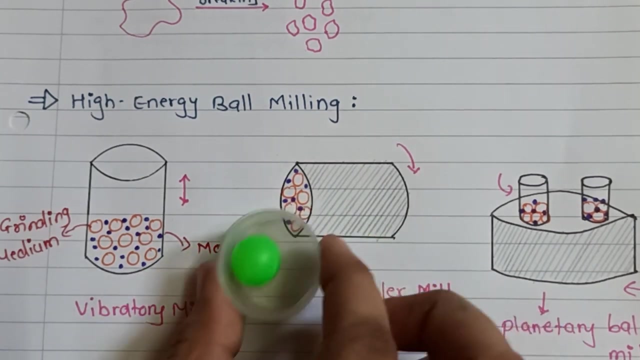 to show all these things. so in this way, we are going to take this wool. what we need to take this wool, that is the nice, which is the still coconut copper clay which is made from donation, that has been self soap and in which salt, so they are going to convert to nanoparticles With the example we use, the. 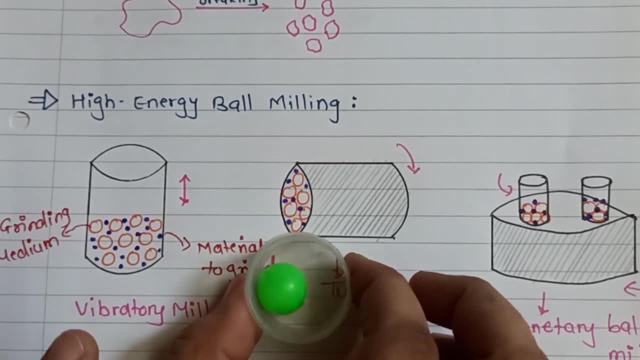 ball better spin this like a na na material. so that is our new, where we put these balls in the mass that we will add into the-a. The collision will be taking place. The collision will be taking place among the. There are several metal balls. Rigid masses will be present. 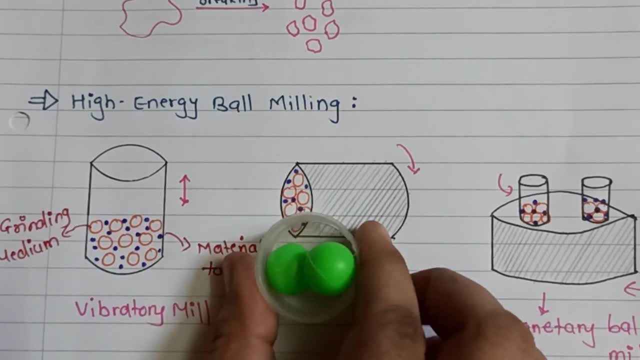 They are going to start to rotating. When they start to rotating, They are collide with itself And collide with the conceal of the container. Collision is happening with the wall of the container. During that, what will happen? The in between the two metal balls, The sample, will start to grind. 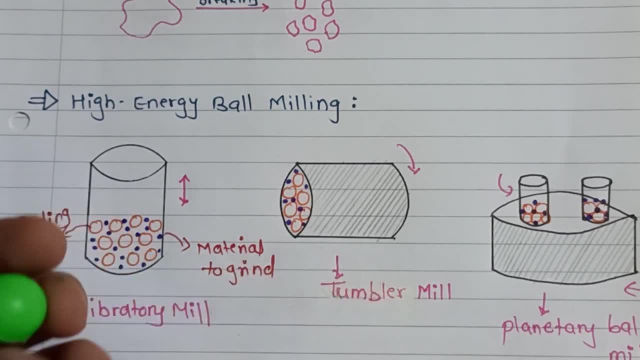 to grind and then they are going to be making the finely powder with the high energy. so these are the actually main process of your what high energy ball milling. that how they are going to be converted into the, your sample, into the nano material. so, as you can see in the all the three, 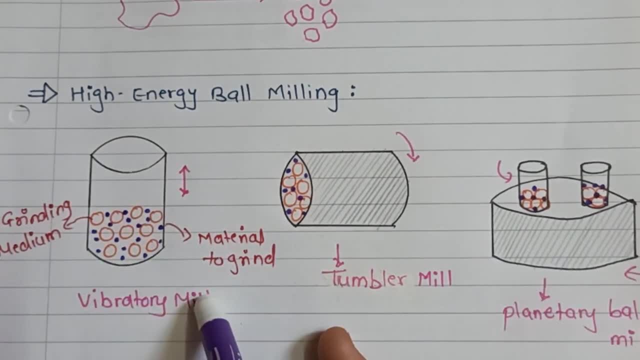 or different kinds of the ball milling. you can see these are the vibratory mill. so what happens here? the vibration will be taking place and during the vibration these are the actually circle which i have made with orange color pencil. that is your grinding medium. so that is stainless steel, or 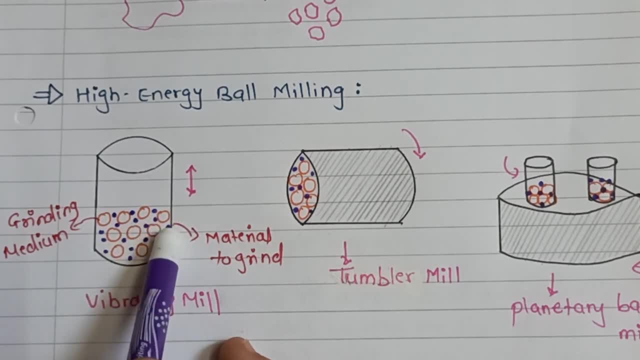 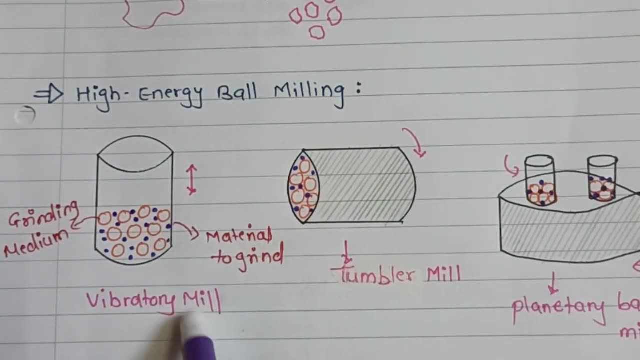 metal body and these are the dotted which i am going to show. the purple color that is your material to grind like we have to make a nano material, then start to vibrate like up down, and then they are going to be creating the what your nano particles. this is the tumbler ball mill. so 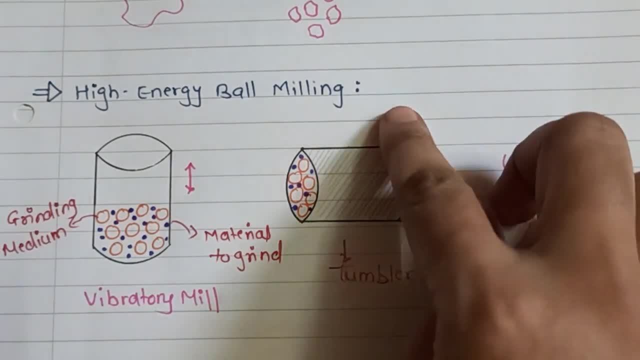 in the tumbler ball mill. they are going to be rotate how? like this. so these are the actually arrow showing you the direction. so it will rotate like this. so, as soon as it will rotate- suppose these are the colors which i have made with the orange color pencil that is your grinding medium. so 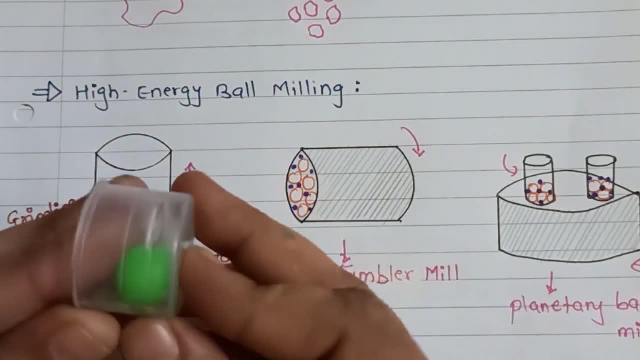 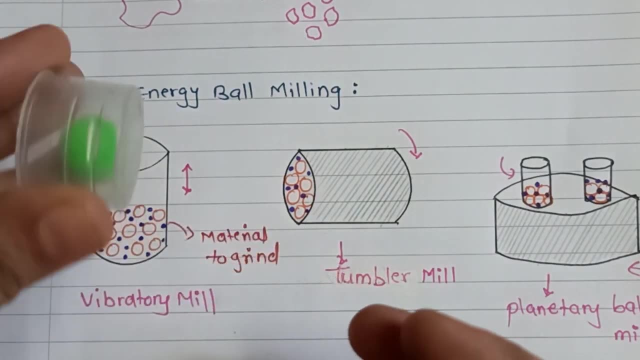 these are the going to be. so it is sealed, okay. and here something is happening. here there is a connection and they are start to rotate like this. so it will be like this. what will happen here? its student will be like this: take a look like this, vertically, they are start to rotate. so this is tumbler ball mill and they 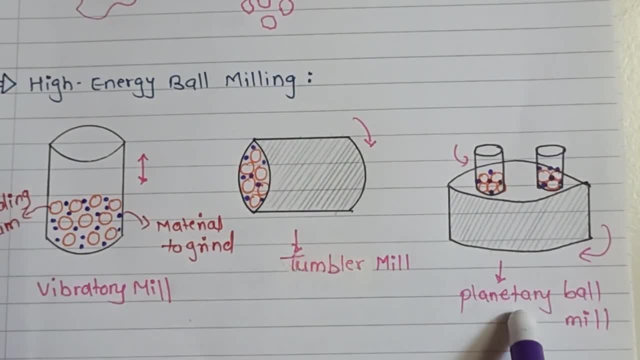 are going to be creating the finely fine powder, and these are the planetary ball mill. the planetary ball mill will rotate like this vessel, whereas the container will be rotated in the opposite direction, and how they are going to be motion into the circular. okay, so this is how we are going to. 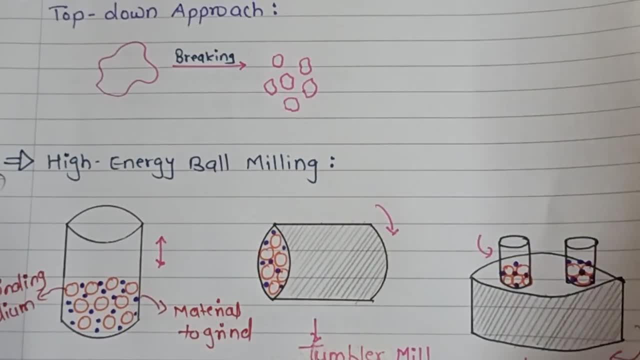 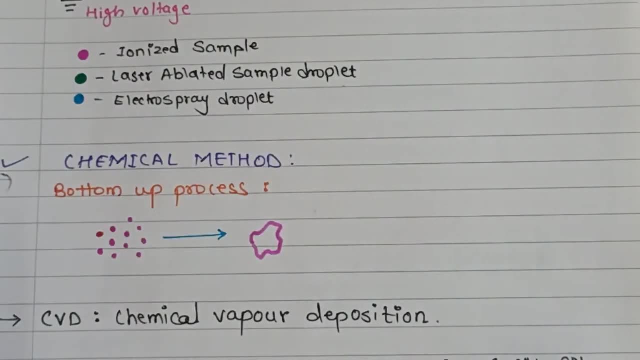 be generating by using the high energy ball milling your nano material. so these are the actually major role of this technique will be the mechanical attrition taking place over here. okay, now, after understand the high energy ball milling, the second one will be the laser ablation method. now, these are the again wafer. 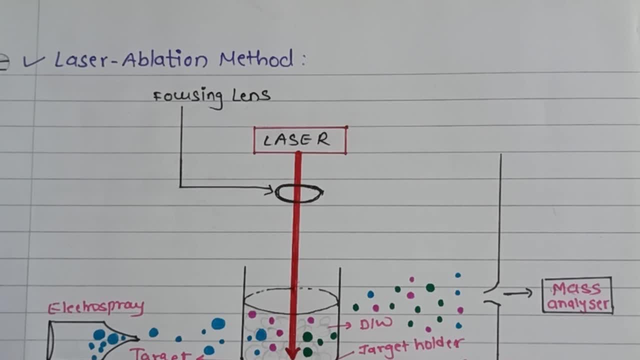 method. now what will be word? obviously here already meno mention kia laser. so laser ka yahape matlabah there will be the some of the light has to be exposure with your. what lights? matlab sample kesad To yahape properlly dethali. 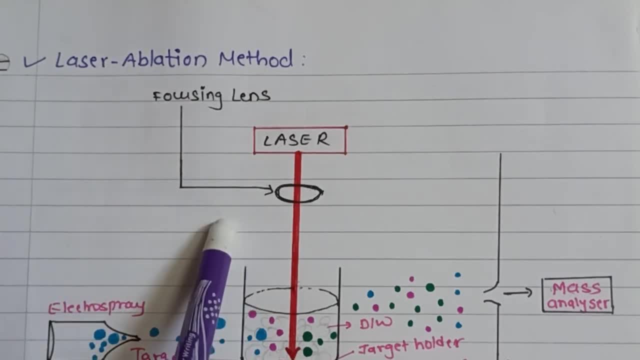 Recently, researchers have developed this laser ablation technique to synthesize nanoparticles of control particle sizes and the composition. So the technique was vaporization of your target using pulse laser. So what we do here is basically we are going to vaporize the target material by using the 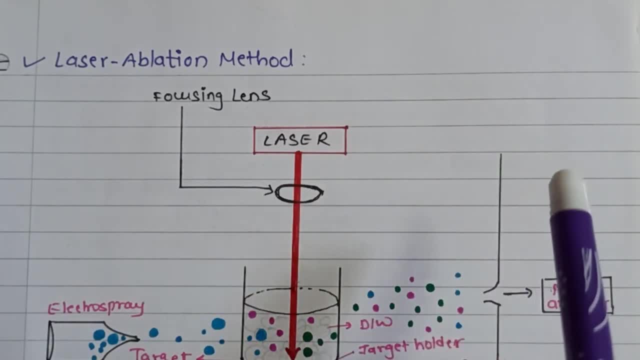 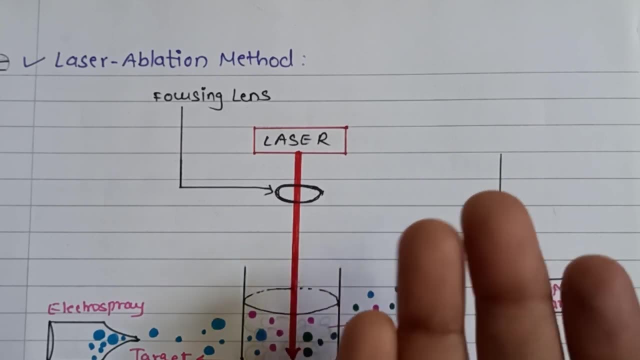 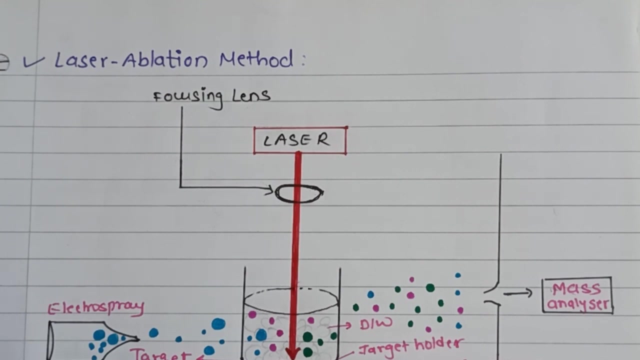 pulse laser and then followed by in the control manner, we are going to condense that material and then finally, in the chamber, or we can say in the container, we will get our interested nanomaterials. So in this method, the vaporization of material are going to be effected by the pulse of the 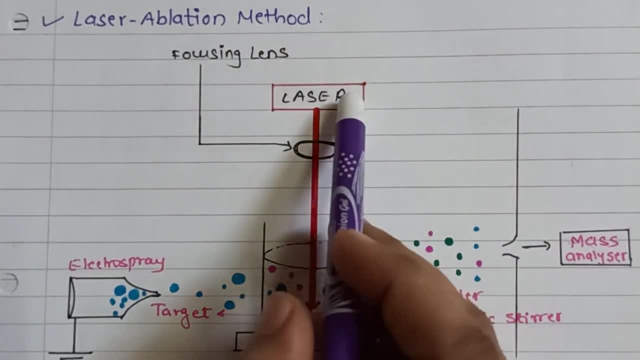 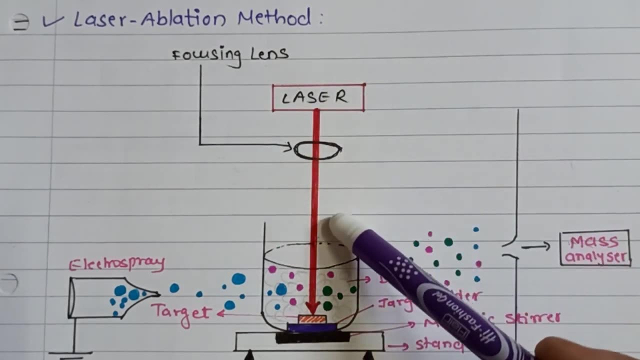 laser beam with the high power. So, as you can see, these are the actually laser light. these are the actually focusing lens. So through these focusing lens, these laser are going to be falls on to your target material. So, as you can see in the complete diagram, these are the actually. your stand here will. 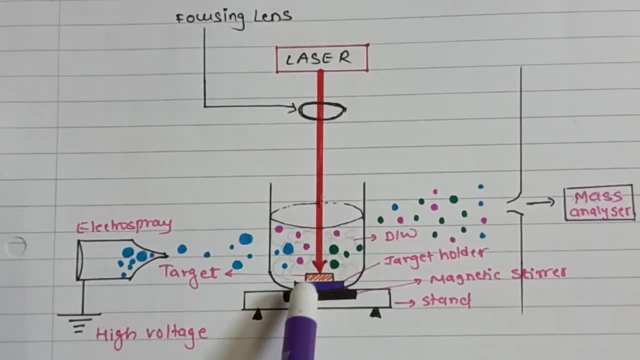 be the mechanics. Terror connection will be there. these are the container. in that container you are going to be, take the distilled water or the nanoparticles or the metal salt. you can say: These are the target holder. on that target holder we are going to place our target. 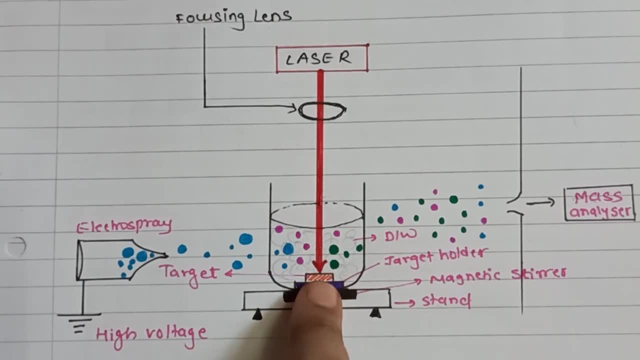 Target means the sample from which we have to make the nanomaterial. So, whichever you are interested to making the nanoparticle, that will be your target Here. you have electrospray. okay, this is connected with the high voltage, and then these are the outlet. 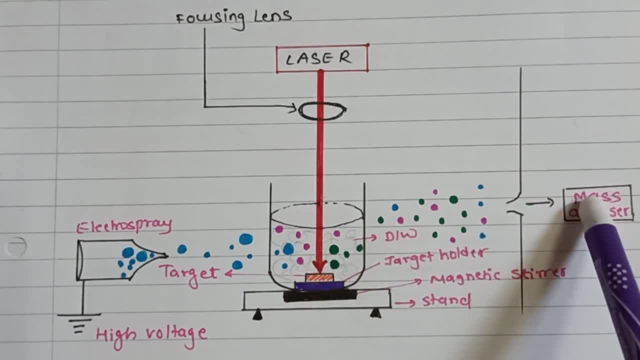 Now, these are the actually coming out, your nanoparticles. Okay, These are the nanoparticles which are going to be coming outside and, with the help of the mass analyzer, we are going to be record the what? your nanomaterials. So we get the data here. 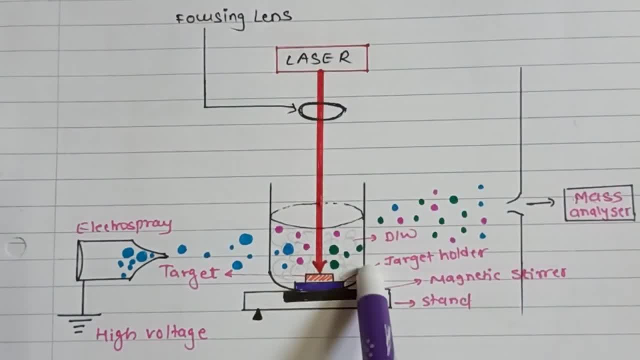 So basically what these laser, as soon as going to be, falls into the, where target material they are going to be, what decompose, they will spread there and they strike to the. then electrons are going to be coming out, and here you can see the three different colors I am: 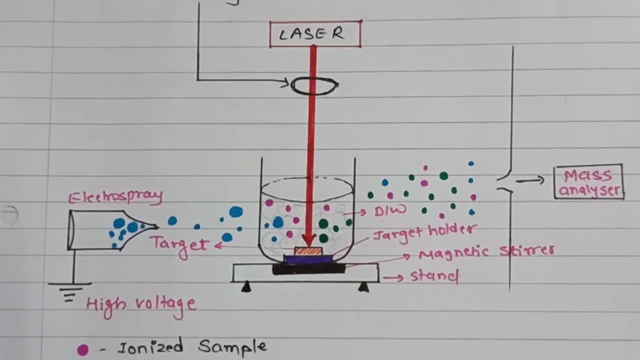 going to be using. So the blue color here, that is your electrospray droplet. they are going to be keeping away the nanoparticles. The green color laser ablated sample droplet now here ablate means student, here see ablater. 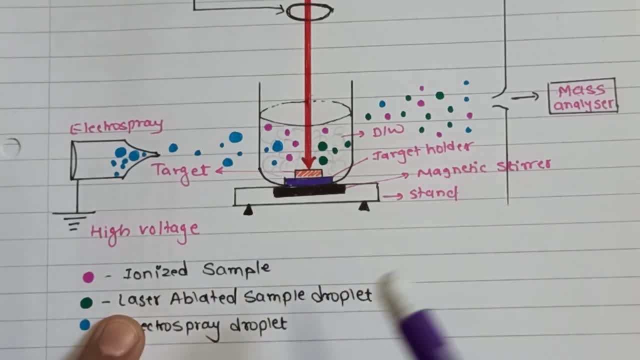 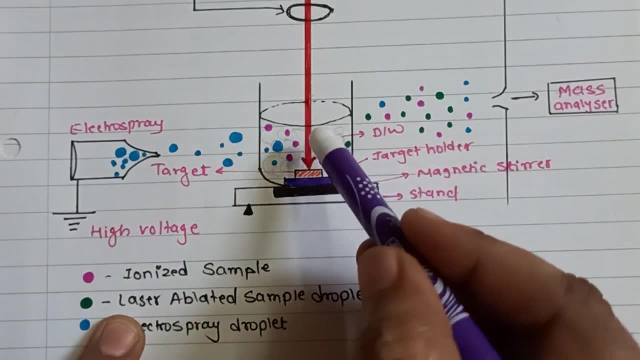 laser. ablated sample droplet means here it happens. ablater means remove what remove. so here the target material is as soon as they are going to be interacted with the laser. so what happens here? immediately the removal of the nanoparticles will be taking place. 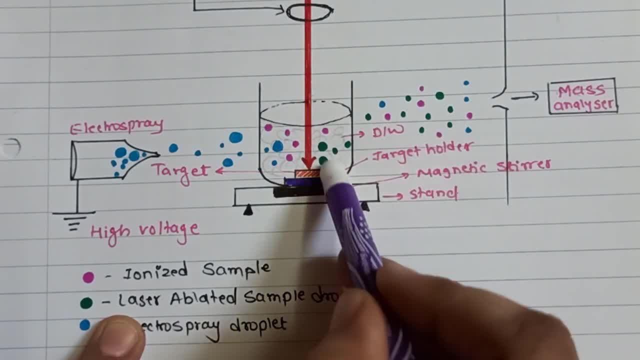 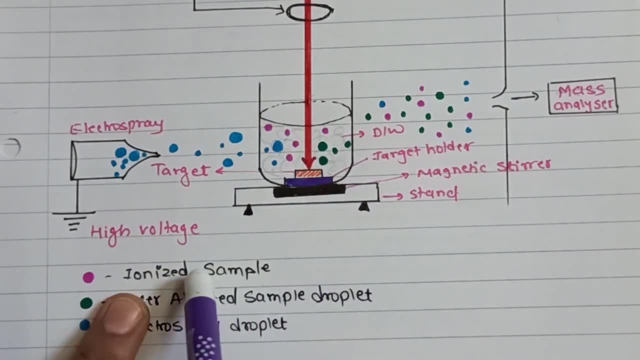 from the sample surface and they are going to be generated as a droplet. so what happens here? their conversion occurs in the nanoparticles After interacting with the laser. Okay, After the interaction with the laser light. and the pink color that I have shown is your. 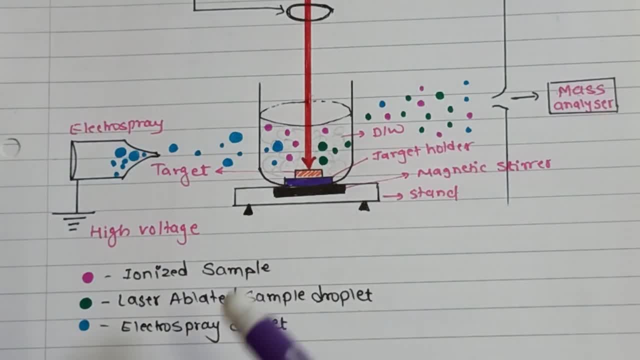 ionized sample. So this is how, after the interaction of the laser, the sample has to be vaporized and generating the nanoparticles that we are going to be connected with the mass analyzer and then, finally, we are going to be detected to it. So these are the- basically what you are- laser ablation method. 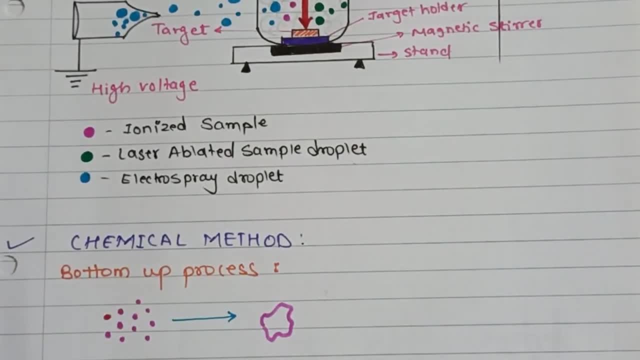 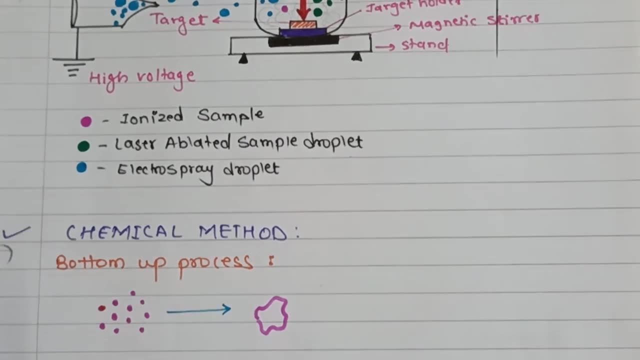 I hope so you should understand it that how we are going to synthesize the nanomaterial. Okay, Now, after understanding both the method, physical laser ablation, and second one will be the high ball milling method. The third method will be your chemical method. 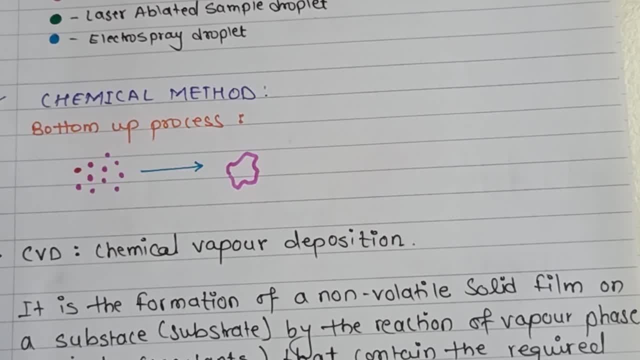 Now chemical method. again, it is about your part of the bottom-up process. Now, bottom-up process is exactly opposite to of your. what top bottom process, a bottom-up process may happen. We are going to consider the smaller molecule over here, Okay, And from that smaller molecule we are going to be combined from the larger molecule. 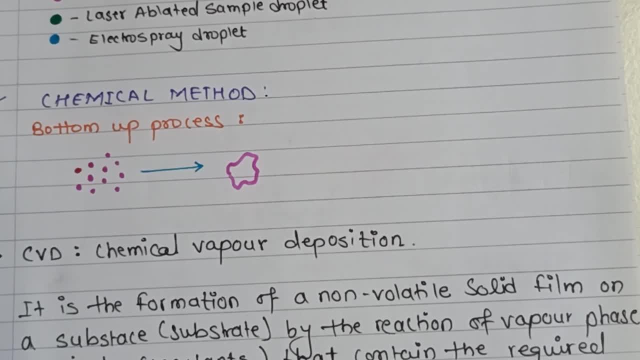 So we call it bottom-up. what process? so in the bottom-up process, okay, the building of nanostructure, We are going to start with the small component, such as atom or the molecules, Okay, which is called as what your bottom-up. So in this method, the raw material sources can be in the form of gas, liquid or the solid. 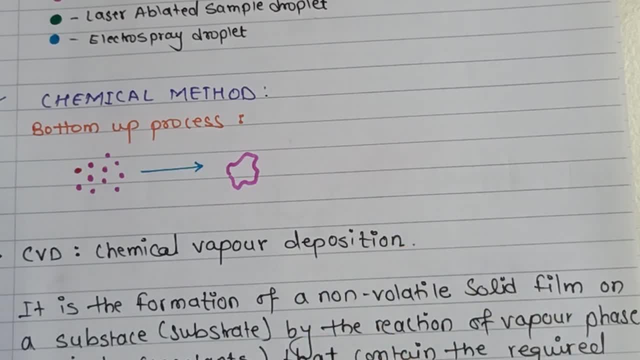 and then later require the some of the sort of the disassembly prior to the incorporation into the nanostructure. Okay, so now we have in the chemical method which we are going to study here- Technique is the first here- CVD. CVD means here chemical vaporization. 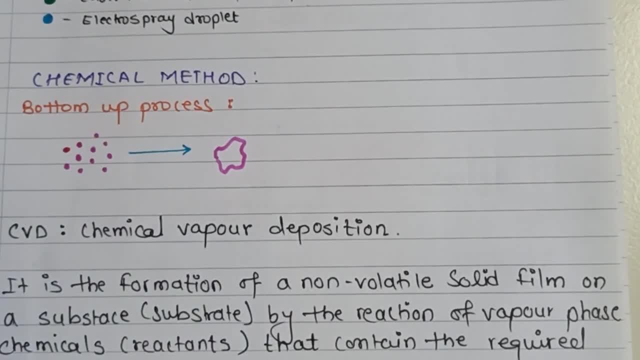 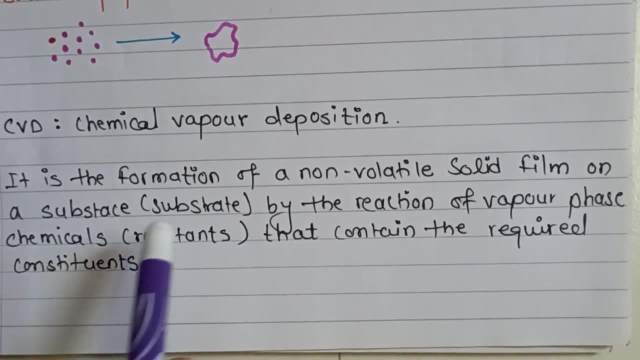 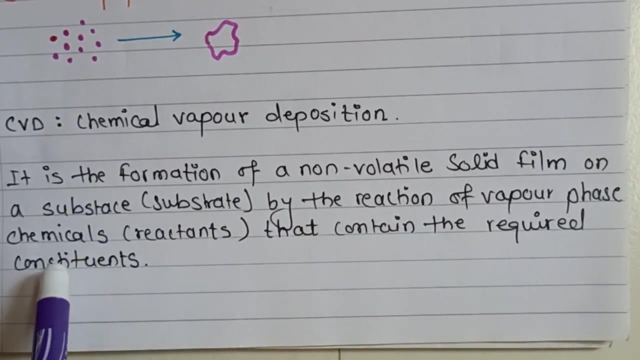 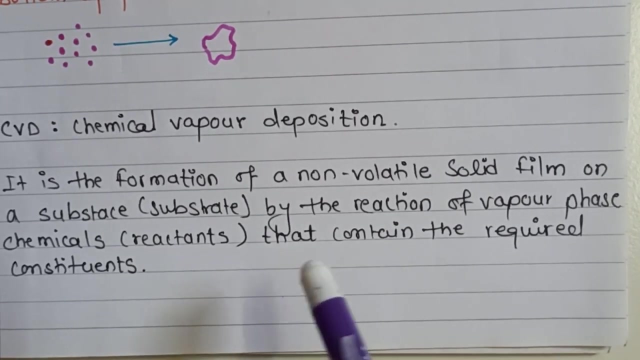 Chemical vaporization. Okay, So what is the meaning over here? So what is the meaning over here? So it is actually formation of non-volatile solid film on a substrate by the reaction of vapor phase chemicals that contain the required contents. So, in short, it is actually a method of the synthesis. 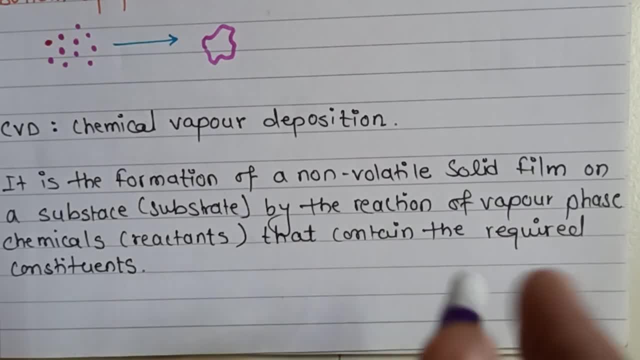 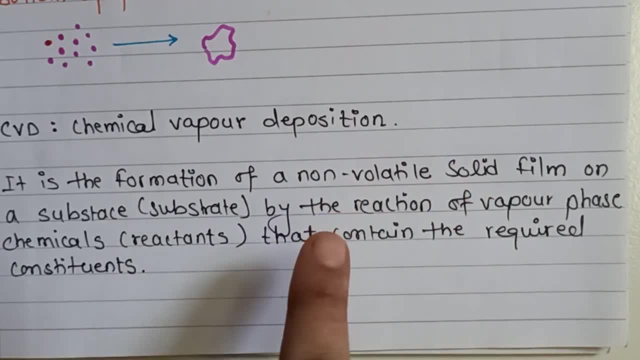 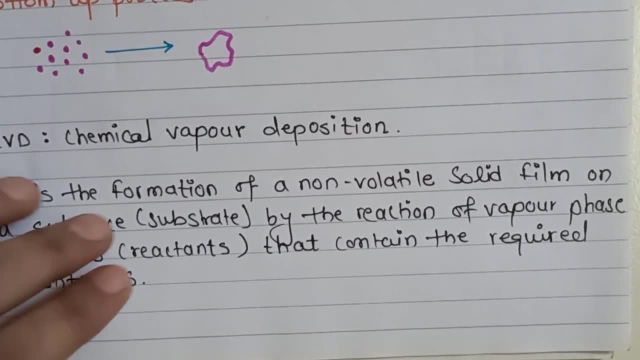 onto the your substances held at the elevated temperature. Now these adsorb molecules are either be thermally decomposed or react with the other gases, and then that vapor to form crystal. So here we are going to follow some step-by-step procedure. 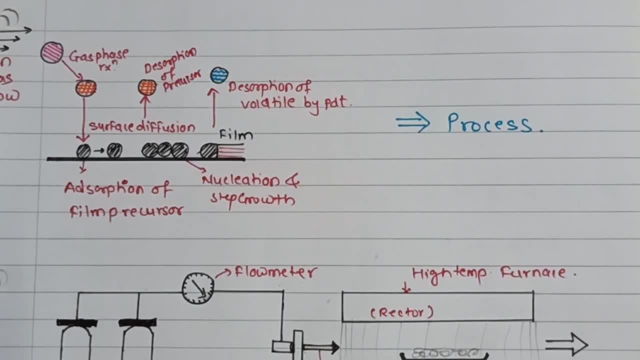 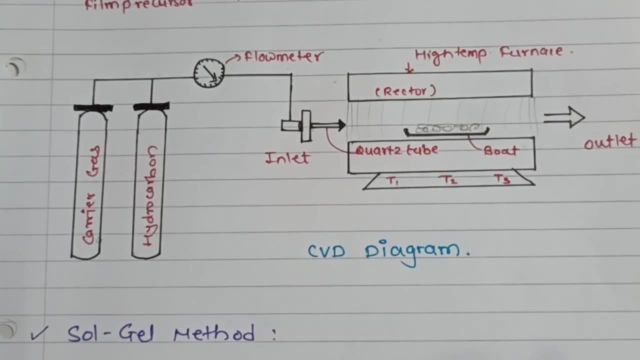 So just take a look in the further diagram I'm just going to be showing over here. So look over here in the diagram, As you can see, these are the main gas flow. First I will show you the diagram of the chemical vapor deposition. 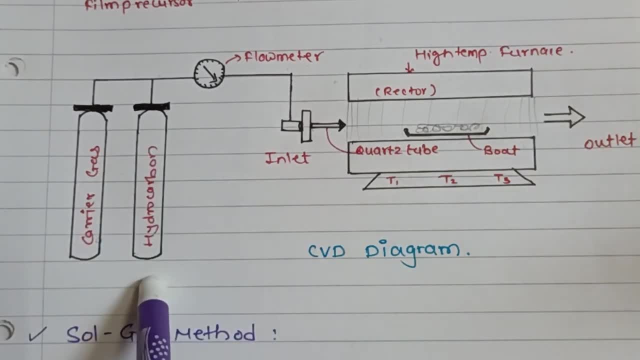 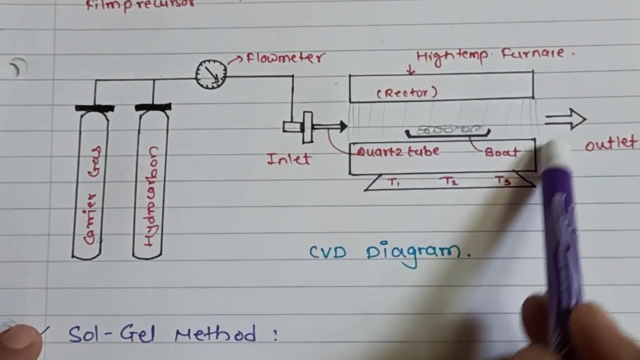 Here are the inlets of the carrier gas and hydrocarbons. These are the flowmeters to maintain the gaseous flow. These are the inlets. The carbon based materials are going to be transported from the inlet. These are the high temperature furnace. This is the furnace body. 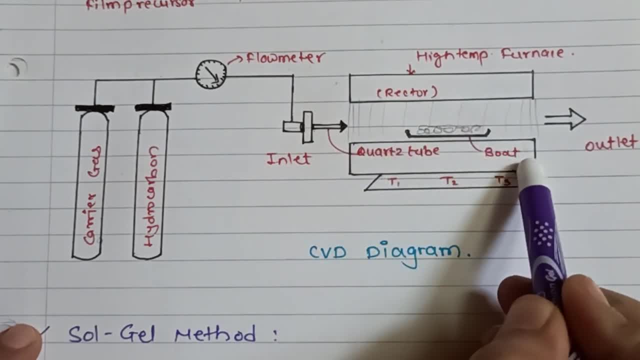 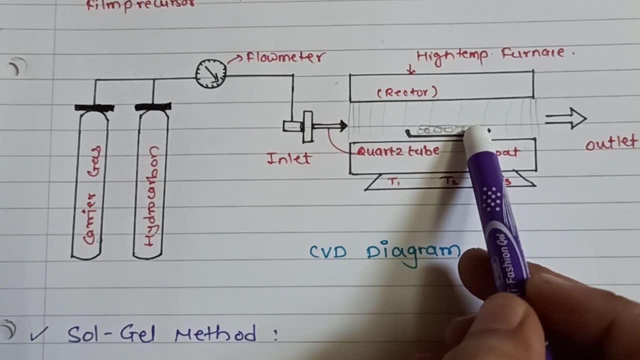 In the middle part of the furnace. Here will be the boat. Here is a flat surface plate. In that place we are going to put our sample. From that we have to generate the nano material. Here will be the sample. These are the quad tube which is connected in the high temperature furnace. 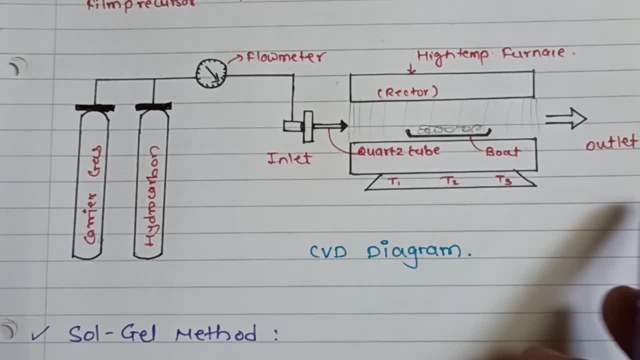 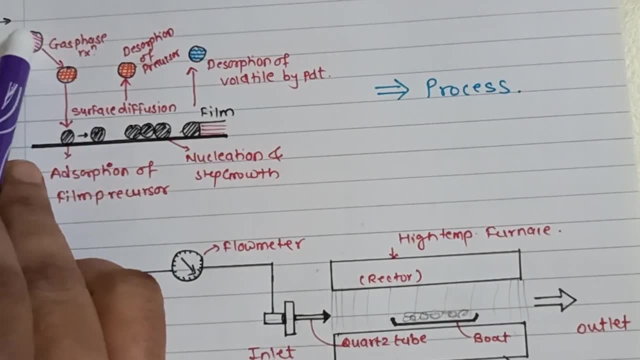 And these are the outlet. Here we can maintain the temperature T1,, T2, T3. As soon as this main gas flow will be started Immediately, the gaseous which are present in the phase reaction, That gaseous phase reaction will be interact. So here, 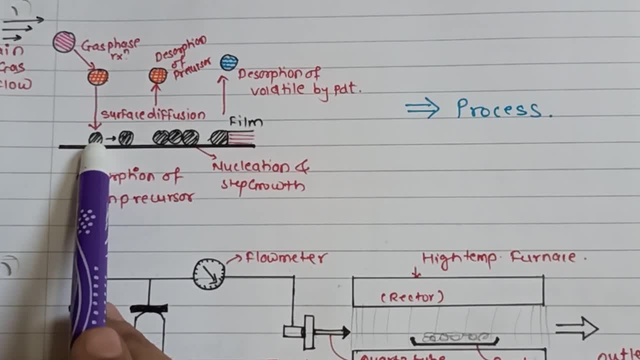 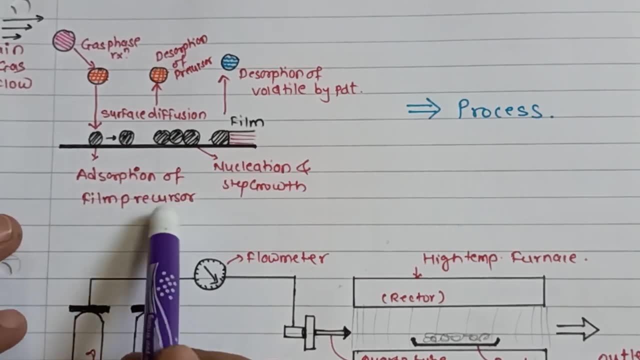 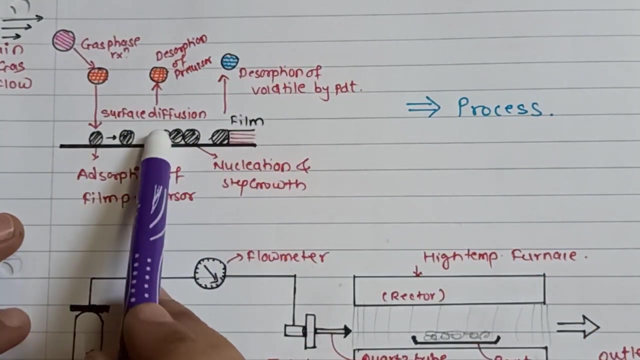 After the carried out the chemical reaction, They are going to be settling down on to the surface, Which is the target material. So here the first step is Adsorption of the film, of the precursor. Then here it happens, Later they are going to be again. This chemical reaction will be continuously started into the chamber. 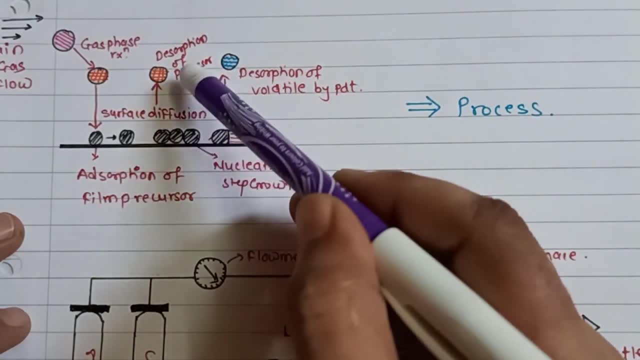 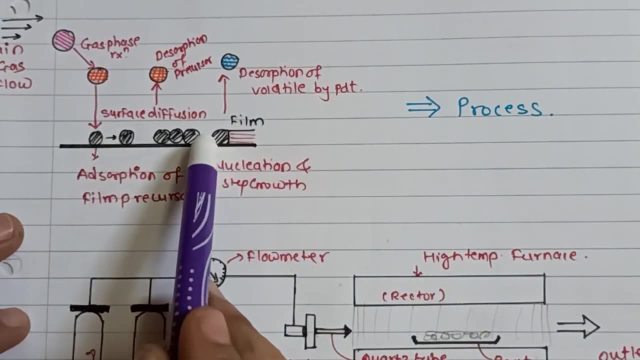 Then further surface diffusion will be taking place. So after surface diffusion, here is the deabsorption of the precursor. So this process will start continuously here. Then, one by one, as you can see over here, One, two, three, four, five, So one by one, this chemical process will be continuously start. 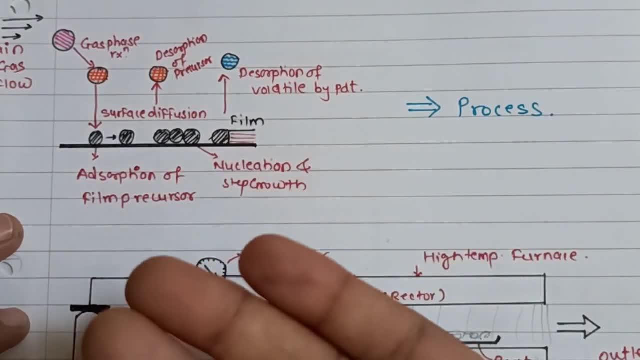 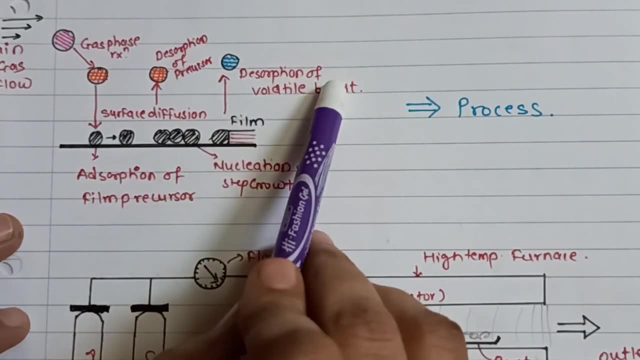 And the one thin film will be here, Generated on to the substrate surface. So this is called nucleation and this step growth, And then this film will be generated And finally, end of the day, The deabsorption of the volatile which is the by-product, Because I had said in the first definition. 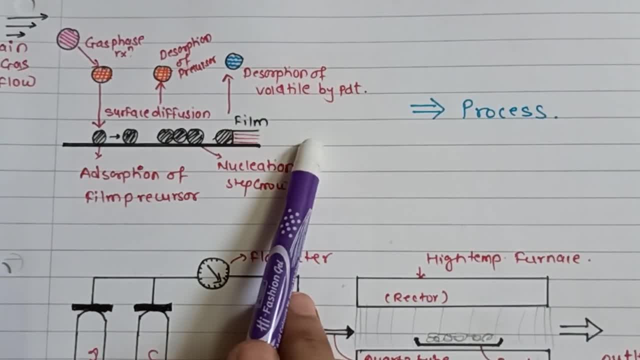 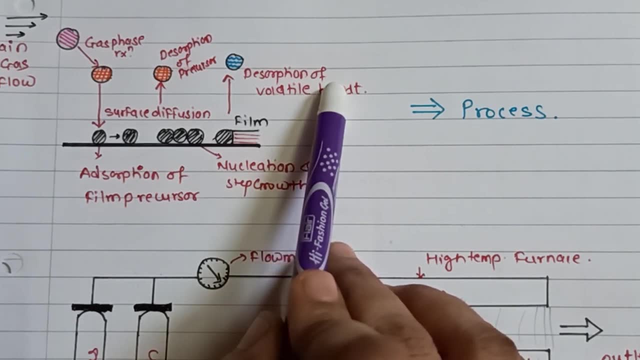 The non-volatile material that has to be. What is the coating here? And the volatile, which is our by-product. What will happen here? Deabsorption will happen. So this is basically what The non-volatile material has to be coated on to the your surface. 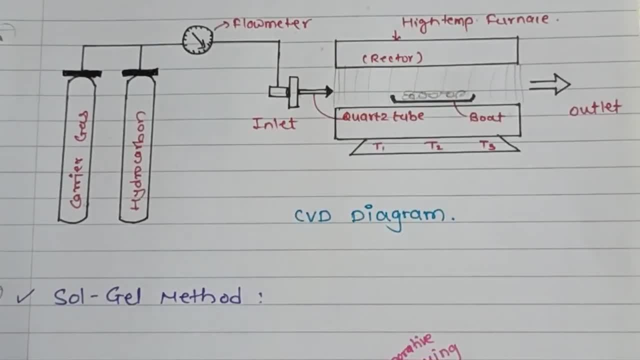 Substrate surface. So we call that chemical vapor deposition. So these are the actually what your whole diagram, So this is the CVD process- will be the more important in point of your formation of the coating. So here the major three processes are. again I am telling The first step is here. 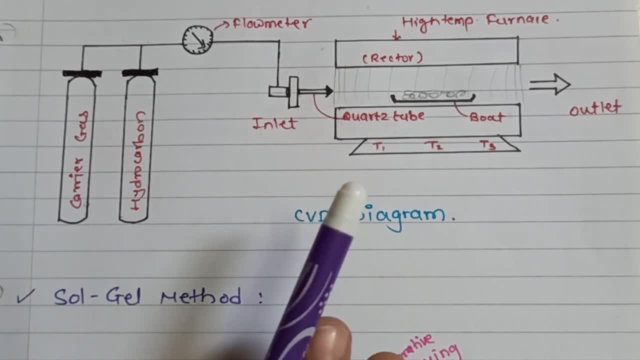 Reactant will move on to the growth surface Via boundary layer diffusion. Second is here: Chemical reaction take place on the growth surface, Okay, And the third will be the Remove of the by-product from the growth surface. So, first of all, what will happen? Growth will happen on the surface, by the diffusion. 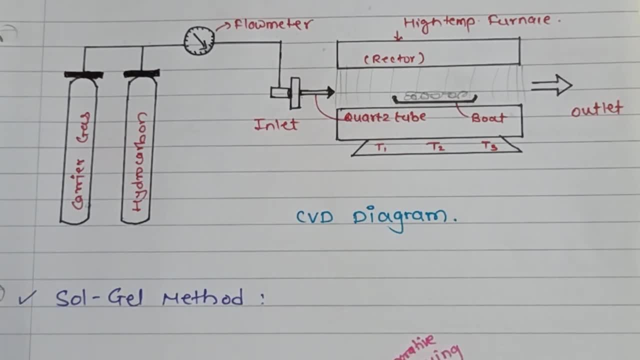 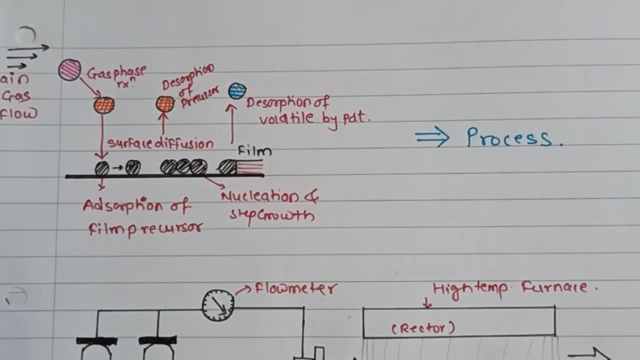 Second Chemical reaction of growth surface And finally, after the reaction, What we have will be the by-product Of the volatile material. What will happen here? Remove will happen. So these are the actually complete diagram of your water CVD, So you can see. these are the chamber Generally here, the temperature of the oven. 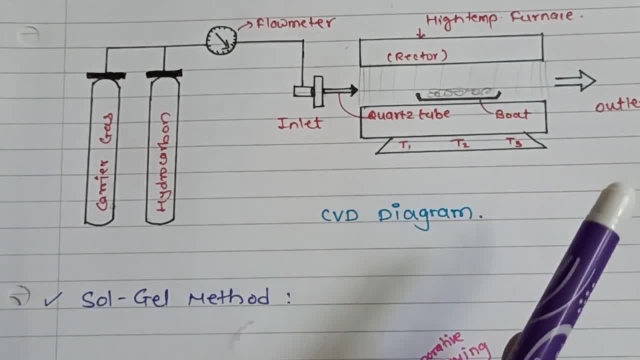 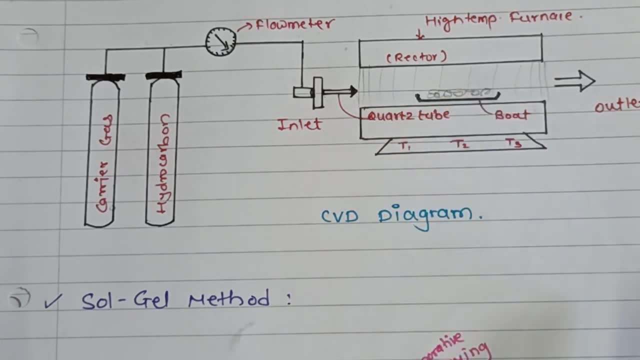 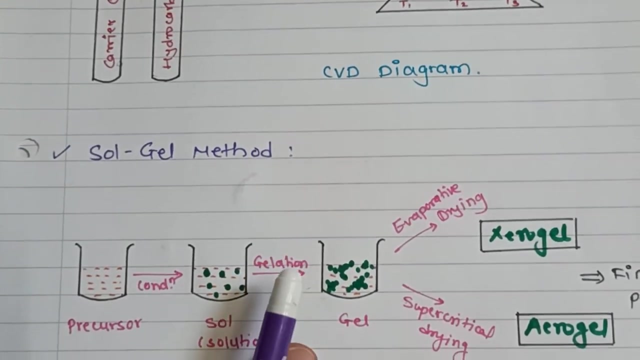 High temperature means 500 to 720 degree Celsius. We maintain the temperature here In between. here, your quartz tube is present here, And in that tube there will be a flat surface on which the sample material will be absorbed by the nanoparticles. Now let's talk about the chemical method, after understanding the CVD. 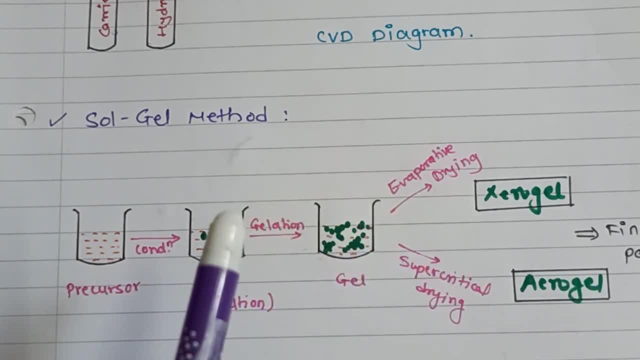 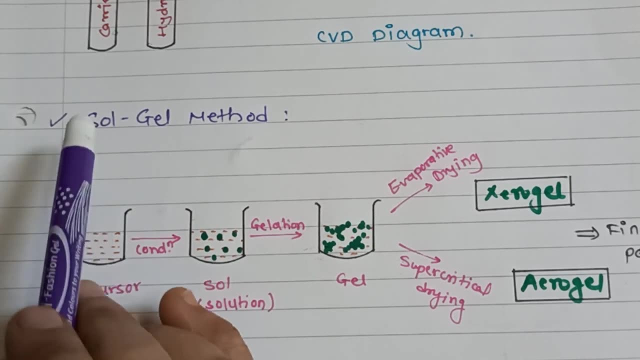 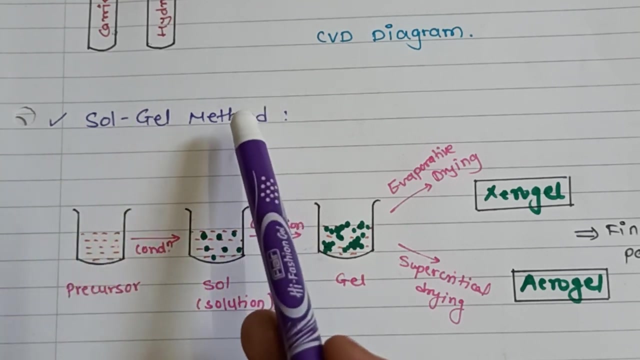 Sol-gel method means. as you can see over here, the word itself is talking about the method. Sol is the one type of the colloidal solution. What is the meaning of gel When the colloidal solution is present in the form of solid or semi-solid form? 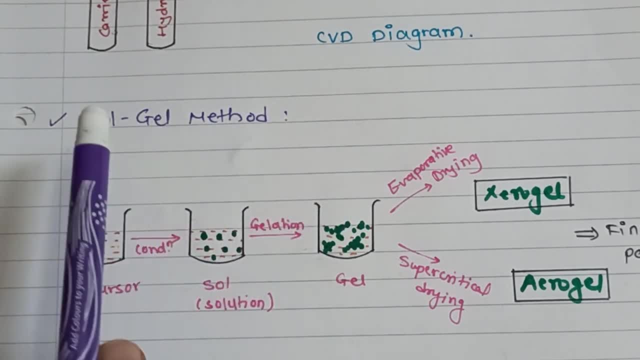 We call it as gel. I hope you know this much. Sol is a colloidal solution Where the gel will be the solid and semi-solid liquid of the colloidal solution. So we can say it is a gel. So first of all, in the Sol-gel method, 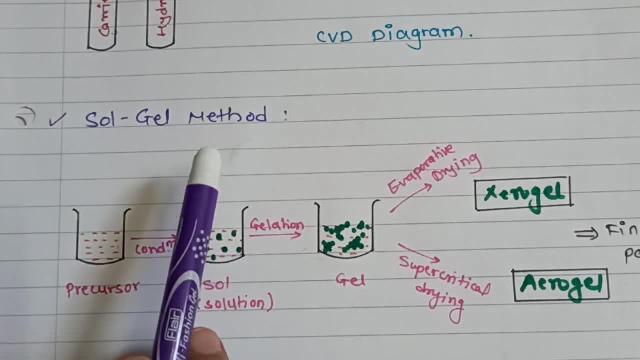 The term is the first time coined in the late 18th And it is actually a low temperature method. This is carried out on the low temperature method, So sometimes This is also called as wet chemical. We can also call this technique. Now, what happens here? first We take the precursor. 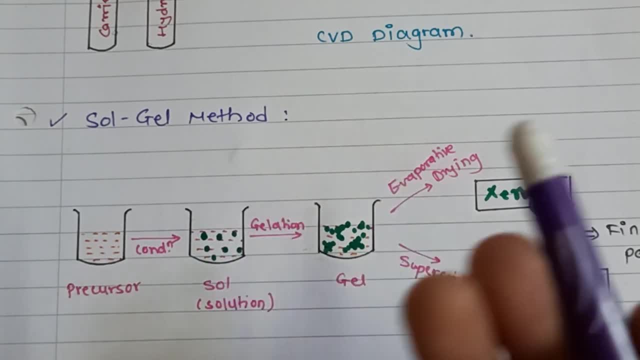 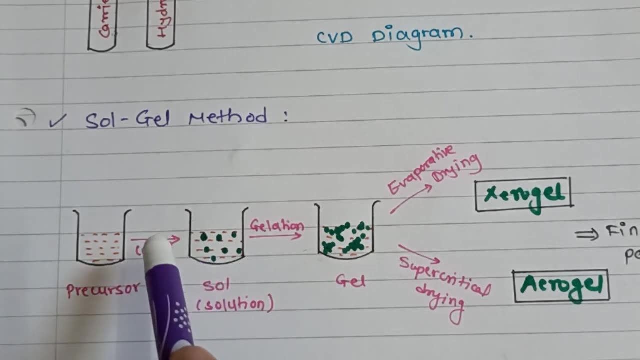 Which we have to make the solution here. So here you will have metal salt nanoparticles. Whichever means you have to make the nanomaterials here, It will be the solution. Then followed that here we start the chemical reaction, Hydrolysis. So here, first, the stirring will be taking place. 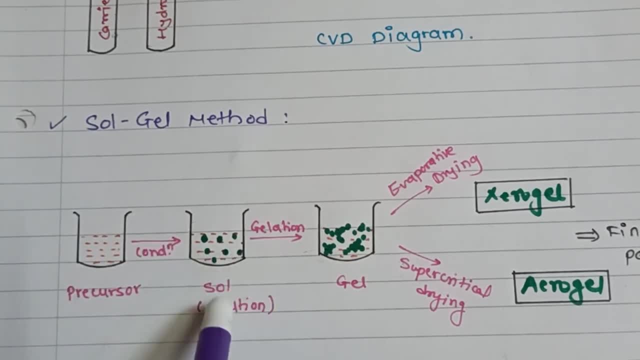 By following the hydrolysis and the condensation Here the Sol will be created. So the Sol formation will be taking place. As you can see In the first beaker and the second beaker You will get the difference. So see here. I have shown the dots of green colour. 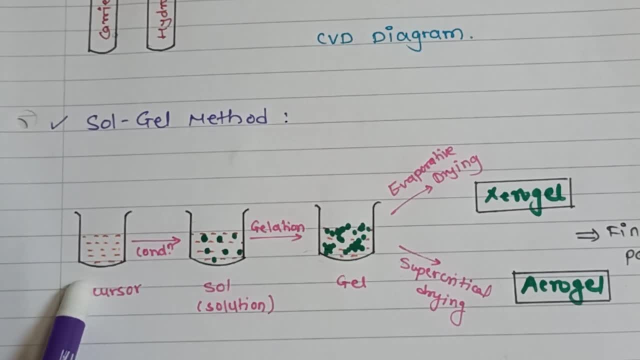 So here you have made the Sol solution. So these are your clear solution. So by following the hydrolysis and the condensation, Now Sol formation will be taking place. Now, after this colloidal solution, The gelation process will be started. So after starting the gelation here, 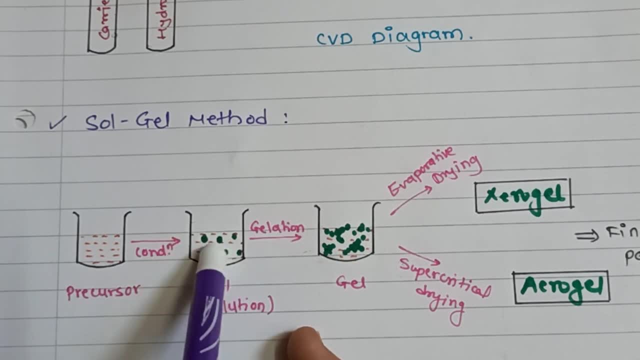 You will get here Integrated network Now all the globules which are visible here, The dots, They are going to be connected. So this is called as integrated network. So here the gel formation will be taking place After the Sol formation And once the Sol and gel, Both the solutions are going to be formed. 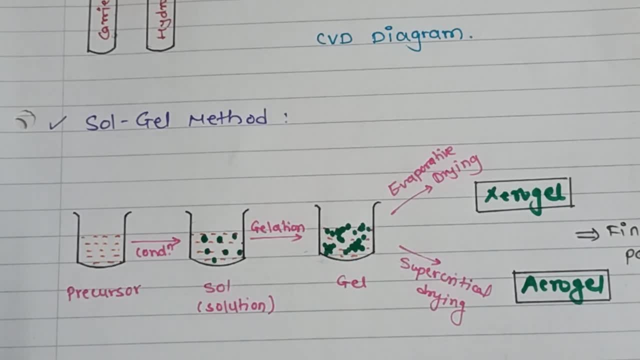 Now this gel will be what your semi-solid solution- Not completely solid- Means. some of the part of the your solid And little part of the liquid will be present. Now this gel has to be drying. So we do the drying process in two ways. First is evaporative drying. 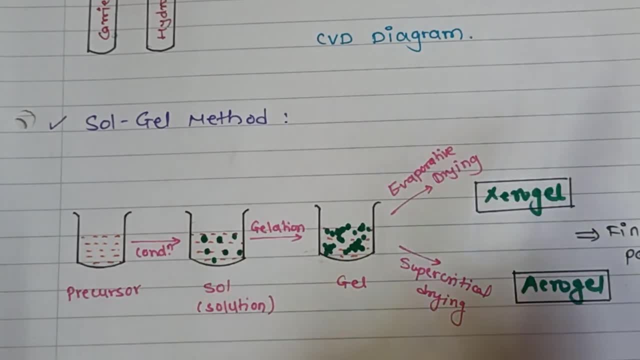 That means we keep the sample in the oven. We will remove the water from it. And second is the drying, And third is the supercritical drying. So once we are going to be if drying the gel In the form of supercritical drying, We will get here aerogel. 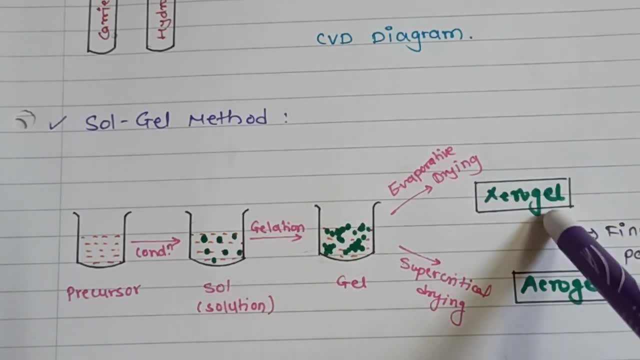 And if we are going to be drying the gel sample By the evaporative drying, So we will get here zero gel And from finally, the zero aerogel, We will get the here final product Means your nano powder And that has to be further characterized And the purification will be taking place. 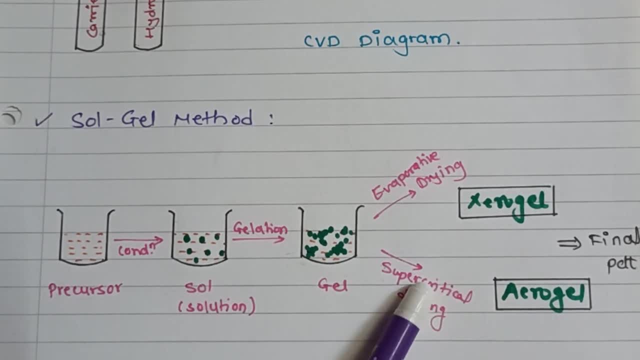 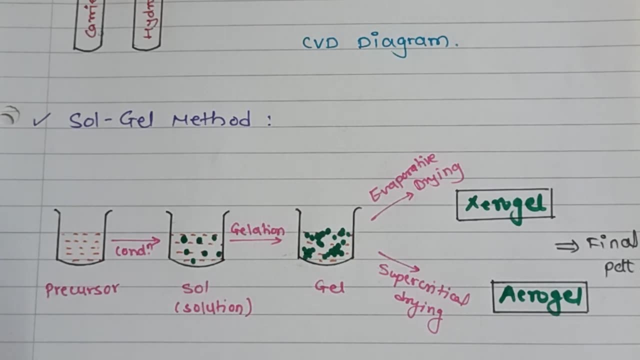 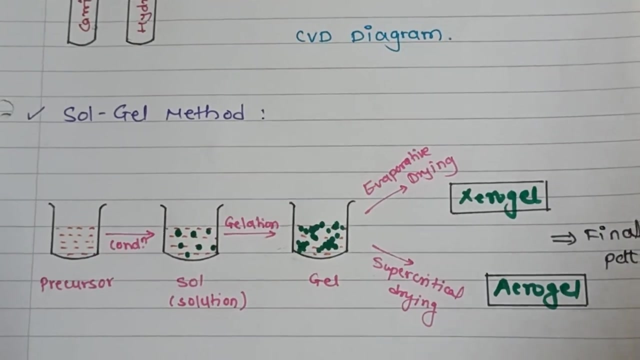 So this is how we are going to be. What synthesize the nano material? By using the Sol gel method. So here, the sol gel method is very famous For metal oxides Like your titanium oxide Or zinc oxide. We can make it very wonderfully By using the sol gel method. 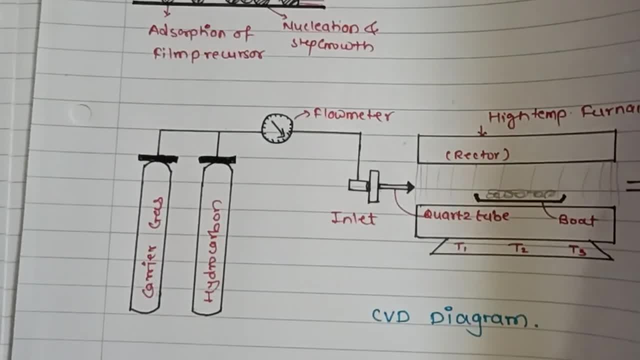 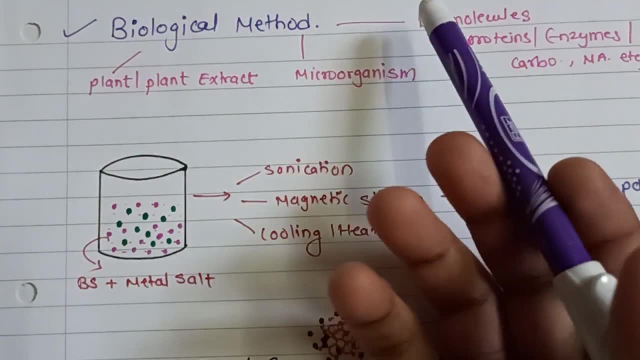 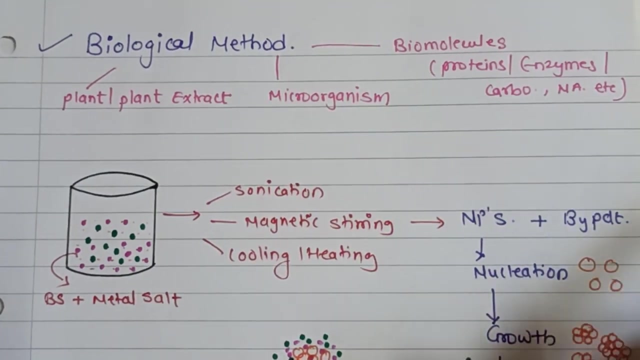 Just, you have to use And you have to see the available chemicals. You have or not. Now, after understanding the chemical method, The last part of this Will be your biological method. Now, biological method means What it is talking about, What your biological ingredient. Now, in this we do three types of study. 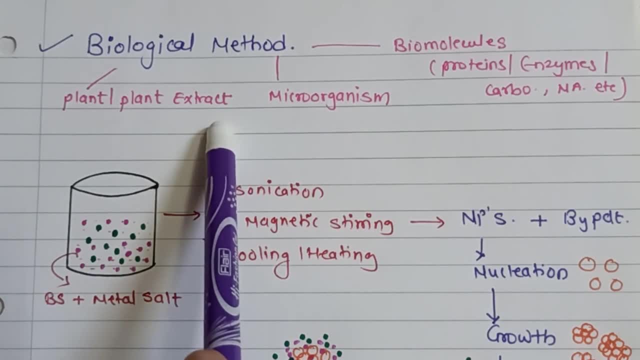 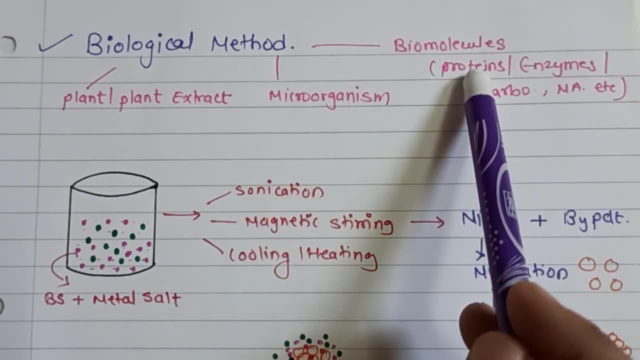 In one biological method. We can use plant or plant extract For the reaction, Or in microorganism- We can take yeast in microorganism, And the bio molecule means We are talking about the proteins, Enzymes, Carbohydrates Or the nucleic acid, etc. So what will happen? 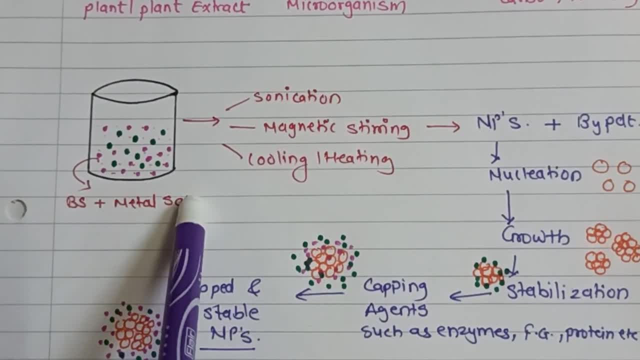 All these biological ingredient. First of all, We are going to be mix with the metal salt. So here, as you can see, These are the dotted Which I have shown: Green and the pink color. These are the what- your biological substances- Along with the metal salt In the container. 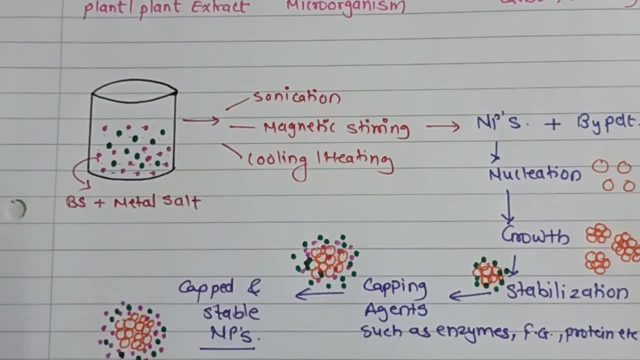 After putting into the container, The reaction will be start. So as what your approach For the chemical reaction, So what we do here, Which nano material we have to make, Depending upon that We are carried out, The first sonication We can do, Or we can do magnetic stir. 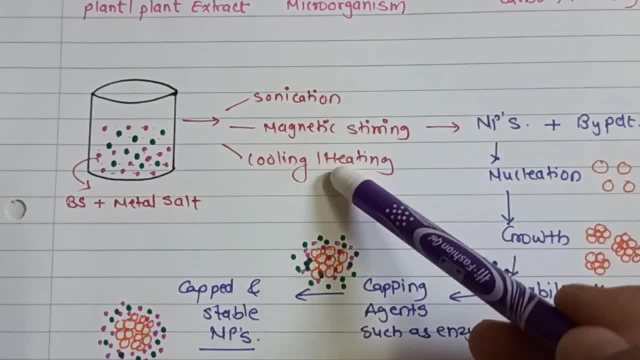 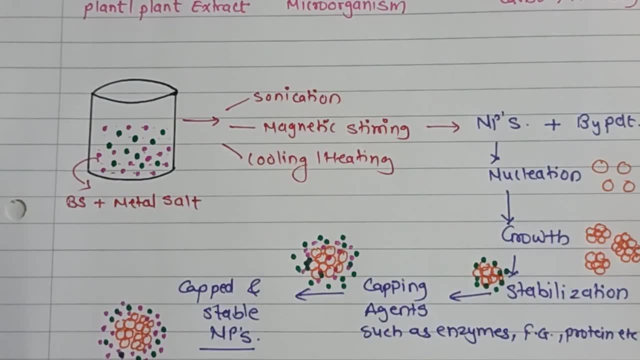 Of the solution Or by following the cooling And the heating technique. So by following the so many processes With the biological substance And the metal salt Get converted into the nano particle. But here your process is not over. After once we will get here By following the one of the process. 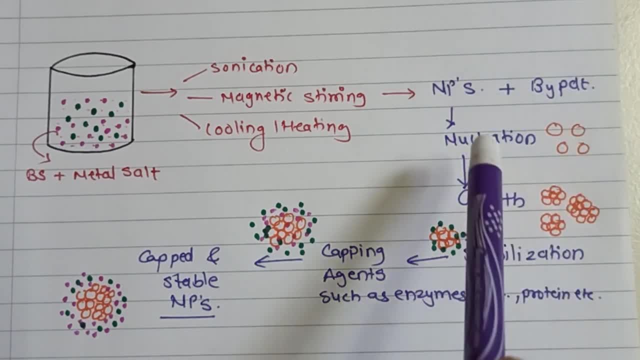 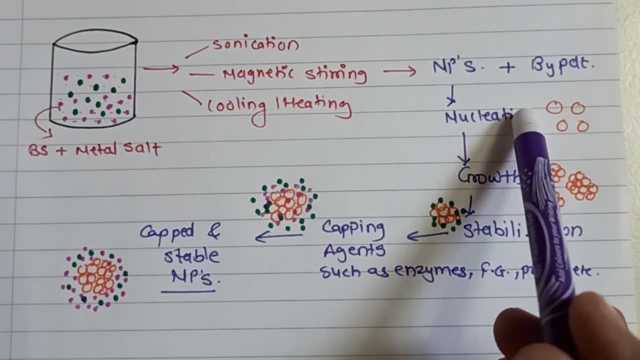 We will get here nano particle Along with the byproduct. Now we remove the byproduct. We are interested into the nano particle. So here you will get single nano particle In the container. Now these nano particle Will be the nucleation. So here their step growth will start. 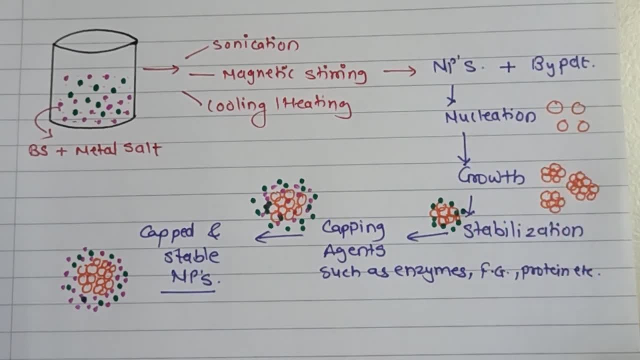 So they are going to be started To combine it together And making the larger molecule. After the growth, Stabilization will be taking place. Now, what is the meaning of stabilization? They are going to be surrounded By the capping agents, Such as the enzymes Functional group of the protein. 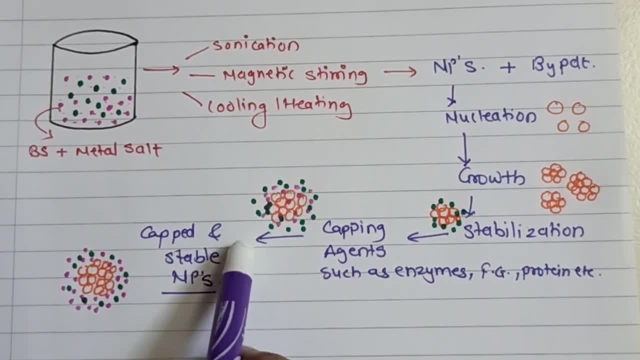 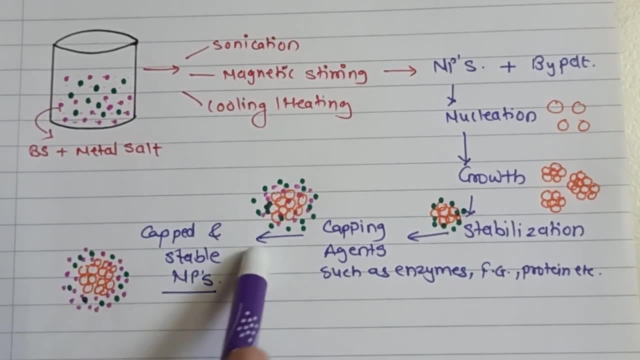 Which ever present into your structure. So they are gives the coating And they are going to be start to stabilize. And finally, we- You will get over here Cap and the stable nano particles, And after getting these stable nano particles, We are going to be purified to it And then further. 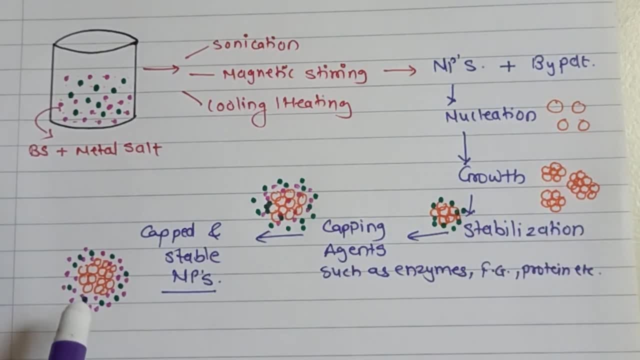 What characterized to it By followed the electron microscopy. Ok, so electron microscopy, You can see the scanning electron microscopy. Then TEMCM log, Because from the visible rays, UV, visible air, We cannot find this nano particles Characterization, So particularly To characterize the nano particle We have to follow. 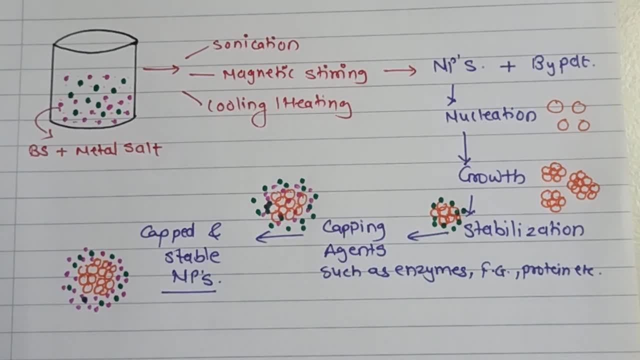 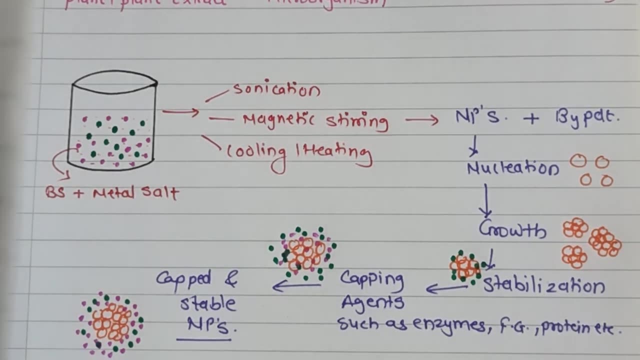 Some of the electron microscopy technique. Ok, So I hope so. student In the all the part, Whatever I am going to be covering In this session, Like your means: introduction Of the nano materials, Then different types of the Your nano materials, Their classification Based on the dimension And finally the synthesis. 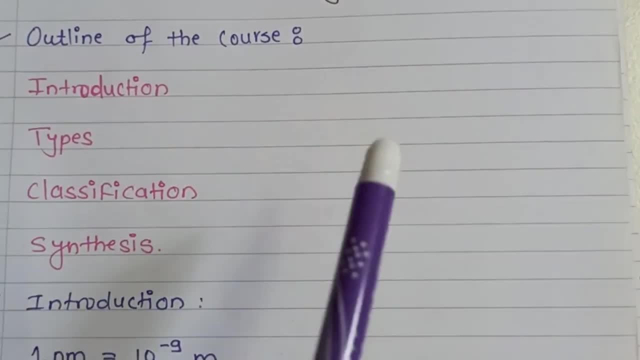 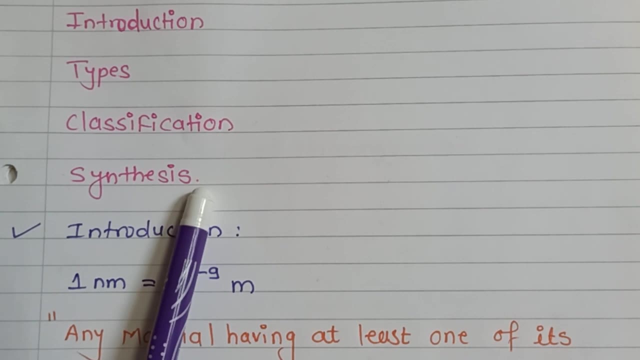 By physical, chemical And the biological method. Ok, I hope so you should clear Your all the considerations. Ok, So I am going to end This session. Thank you very much For your attention. Thank you, Bye, bye, Bye, bye. Good luck Now, guys. I hope you guys Had a good meeting.